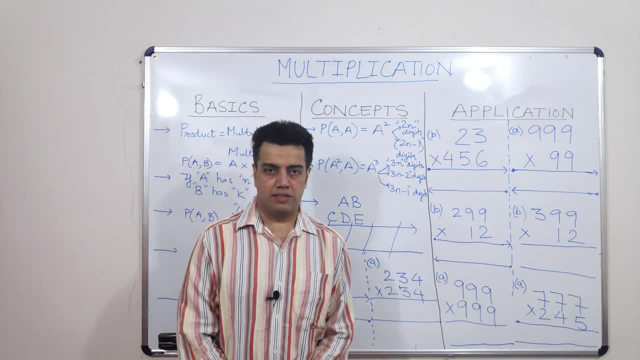 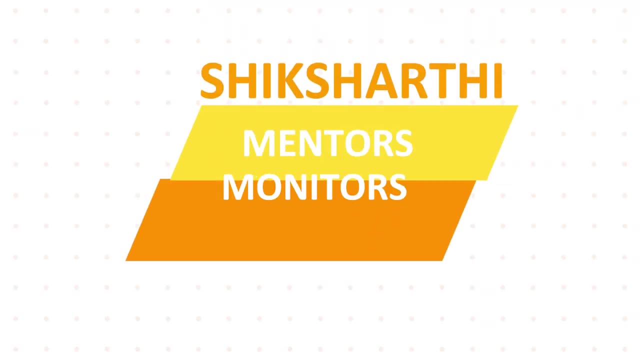 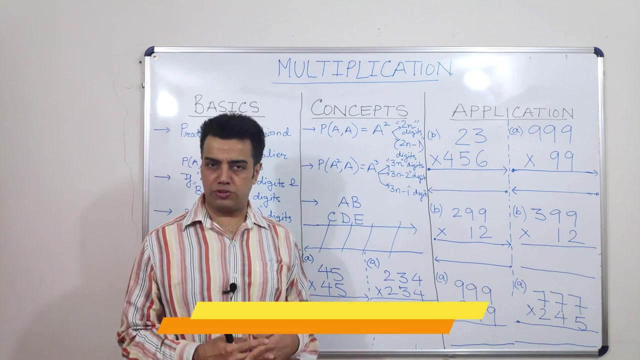 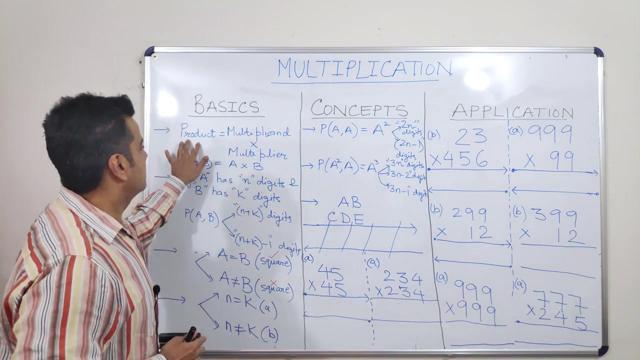 Hello friends, welcome to Shikshati. In this session, we will be taking the topic multiplications to the next level. Now, when I say that I will be taking the topic multiplications to the next level, what do I mean basically is we all are aware of the fact that product is 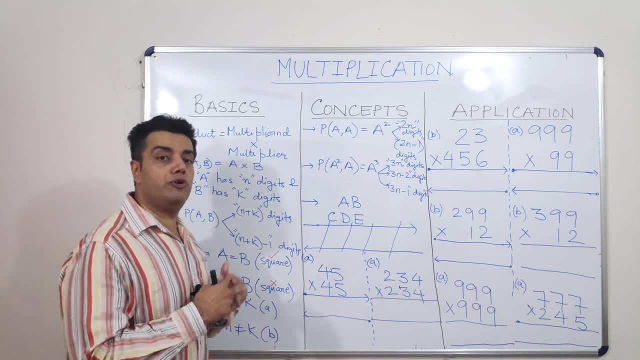 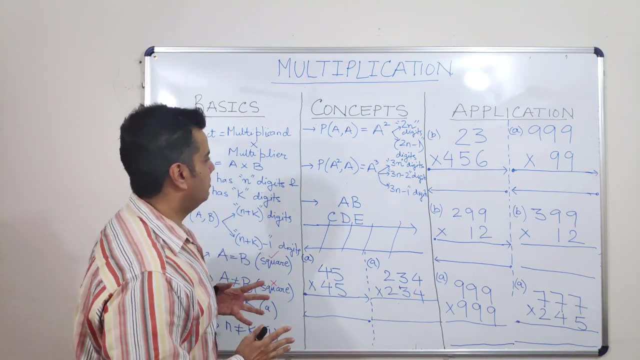 equal to a multiplicant into a multiplier. Before we begin, I would again divide this session into three parts. These three parts would be: we will be discussing the basics, then we will build up the basics with the help of concepts. Now, while we are building, 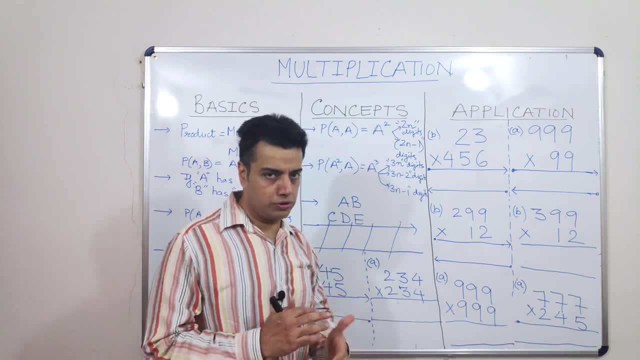 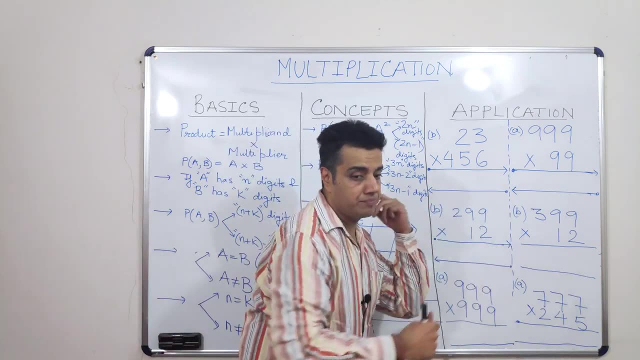 up the concepts. we will be practicing some concepts also, which is equally important, And finally, we will be taking the basics and the concepts to the application level. Now, when I say that I will be taking the basics and the concepts to the application level, The concepts do talk about the basics. 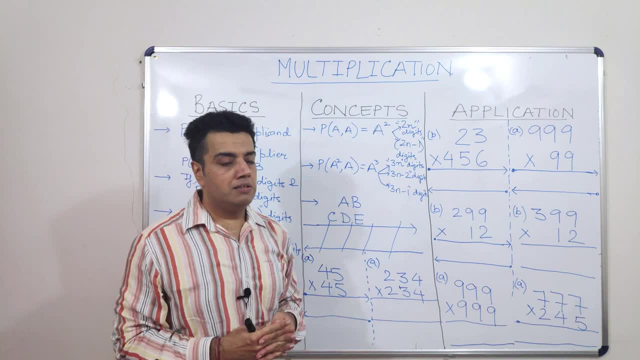 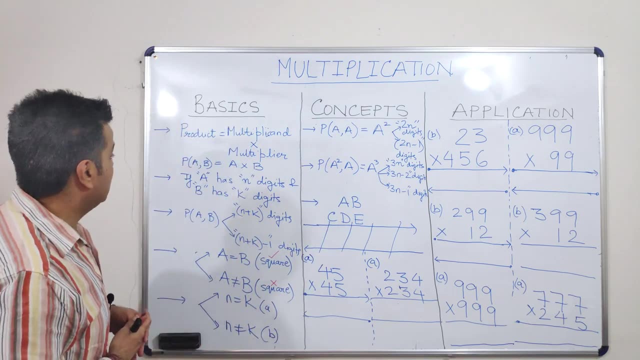 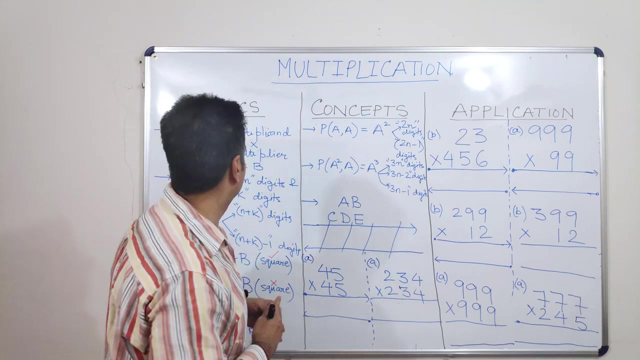 and concepts to the application level. what do i mean to say? is practice makes one perfect? i mean we need to practice as well. so let's come back. so, as i was saying, a product is equal to a multiplicand into a multiplier. all of us are aware of this. now, if i say product of a given number, 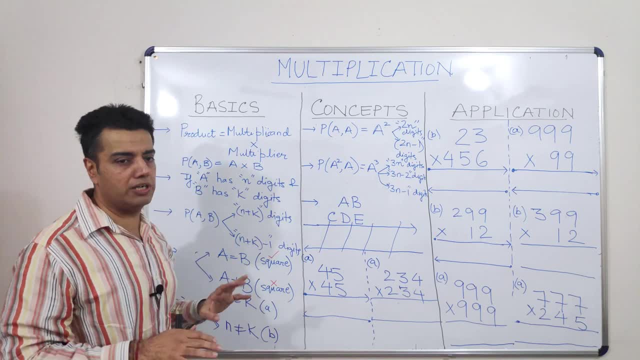 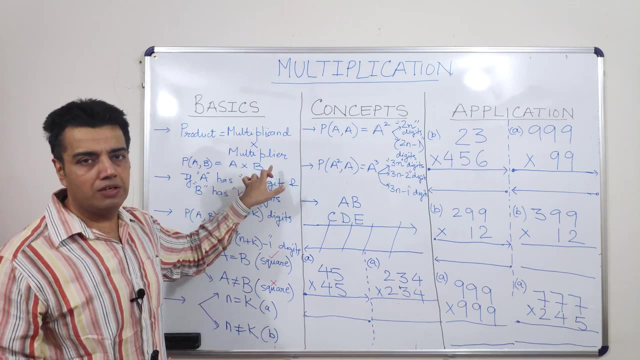 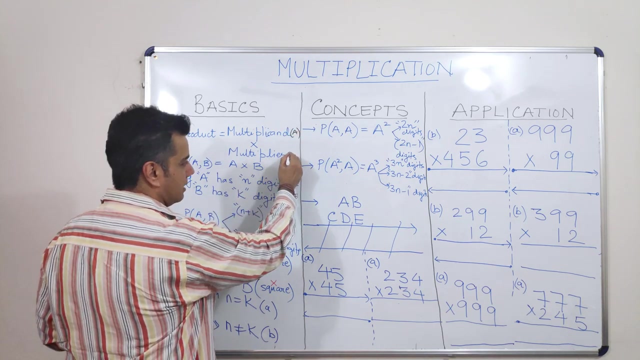 is, let's say, product of two given numbers, is denoted by product of a comma b. now, product of a comma b means that i am taking the product of a with b or b with a. now, in this case i have assumed that the multiplicand is a and the multiplier is b. 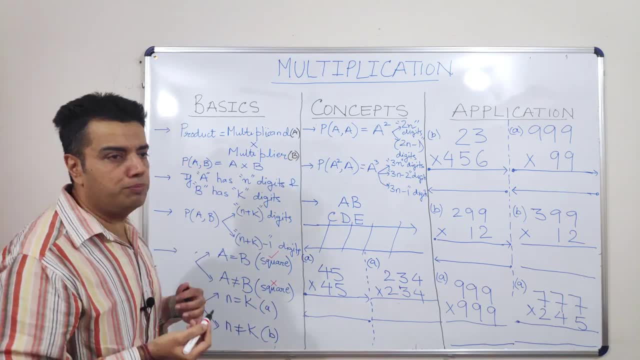 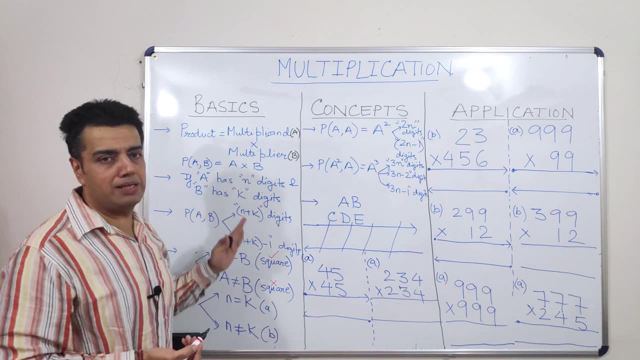 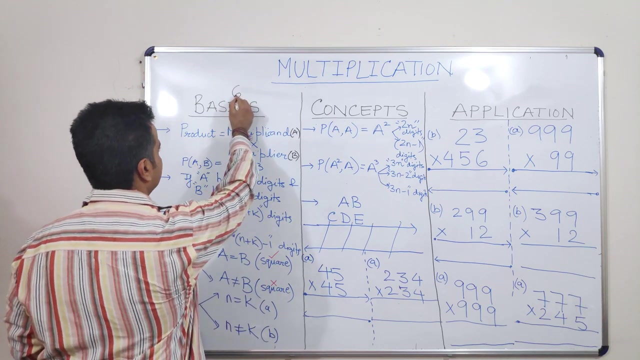 right. i hope you are aware of the fact that the multiplier always comes thereafter. i mean first, you would always like write the multiplicand followed by the multiplier. i mean, if i were to take an example for this, if i take a number like six and if i write it as two into three, then this is the value of a and this is the value of b. 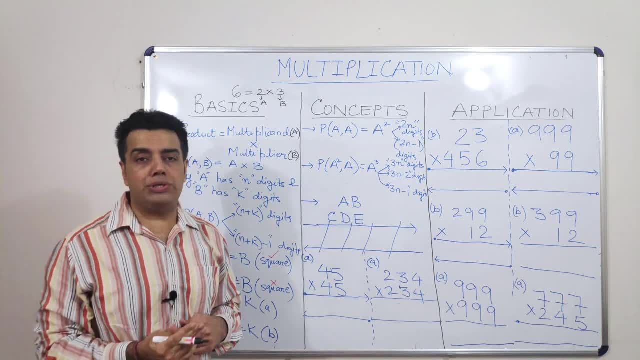 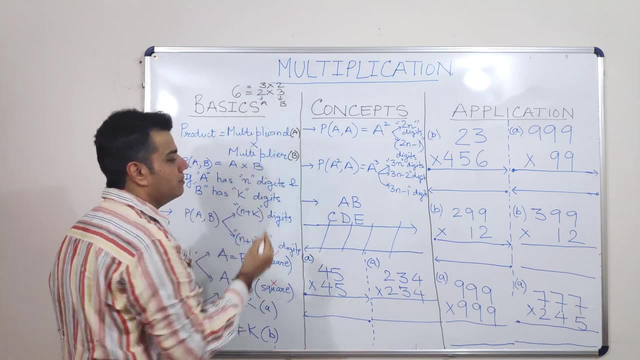 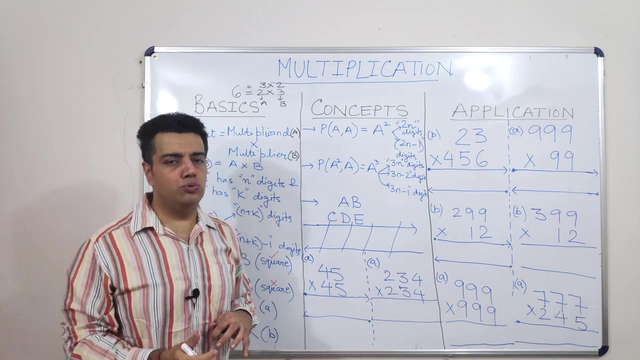 which means two is the multiplicand and three is the multiplier. the same thing. i can write it like three into two also nonetheless, but in that case the multiplier becomes a two and the multiplicand becomes a three. in any case, whether i take the multiplier or the multiplicand as two, 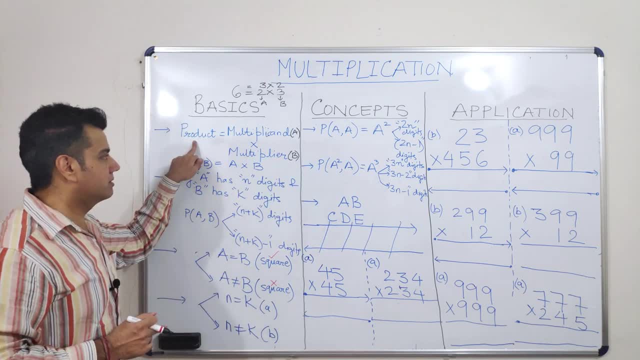 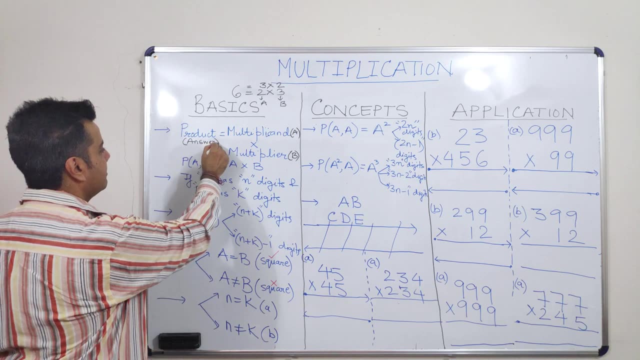 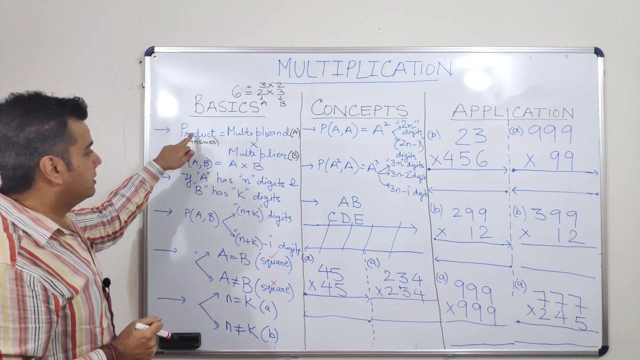 the answer has to be a six. now, what is the answer? the product. so in a certain way, the product is nothing but the answer when two numbers are multiplied with each other. now taking this to the next level. so now, in this number, this product, the number here. 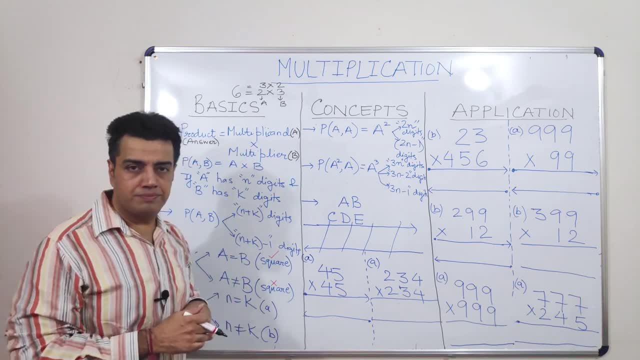 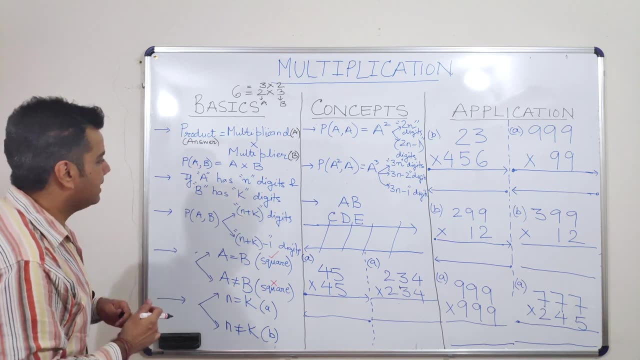 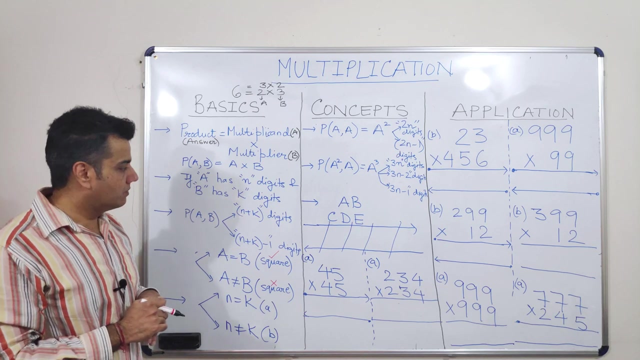 let us say the multiplicand has n digits and the multiplier, which is b, has k digits. so the next basics that i am going to discuss here is the product here will have how many digits. so if i say the product here will have either n plus k digits, 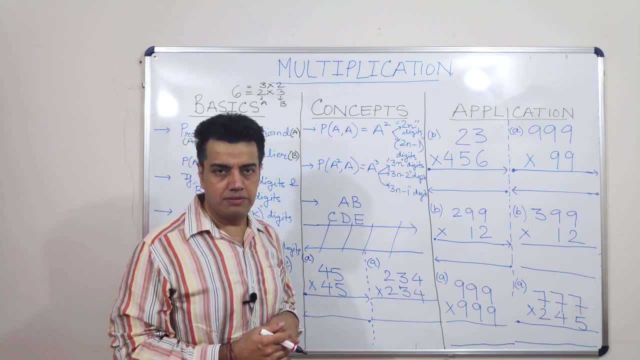 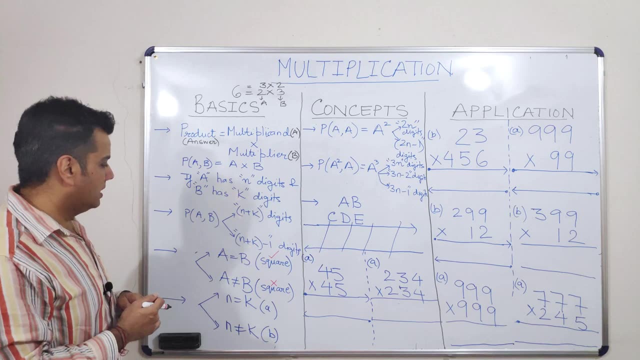 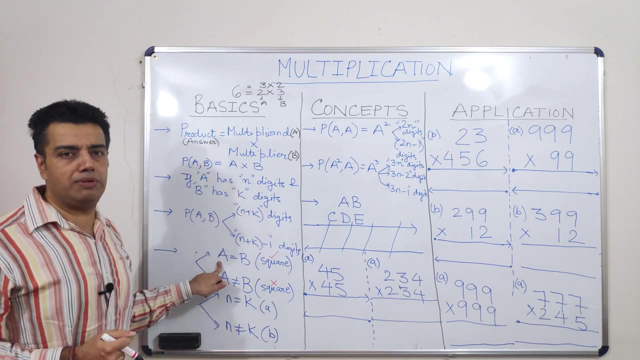 or n plus k minus 1 digits. right, so we will discuss this with the help of few examples. next, when i take this discussion forward, when i am taking a product of two numbers, there may be a possibility that both the numbers are the same. there may be a possibility that both. 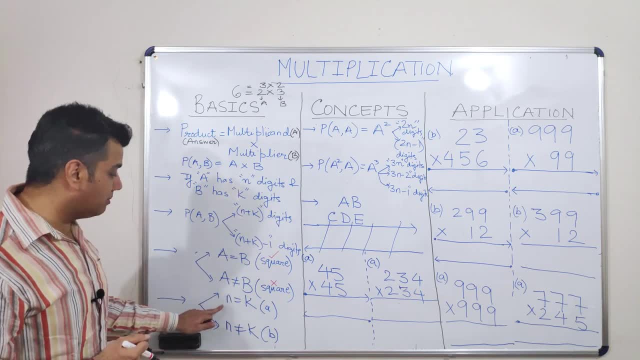 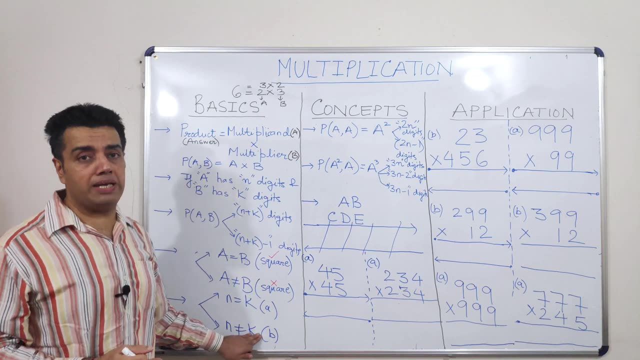 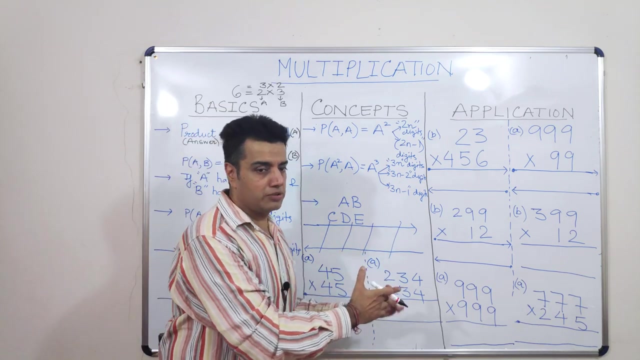 the numbers may be different. there may be a possibility that the number of digits in both the numbers are the same. there may be a possibility that both the numbers may have different digits- confused. oh, it's time to now build up your basics. so, as discussed earlier, this is the element of theory which we call it as basics. now, when i take these, 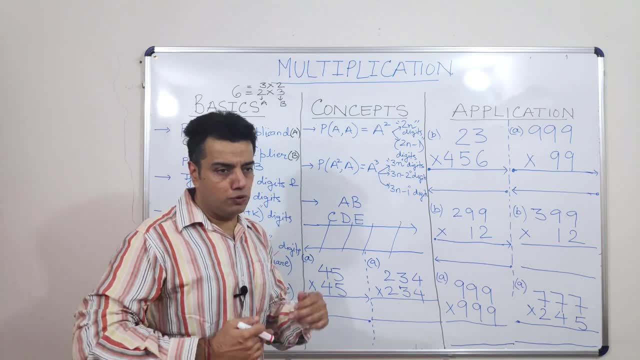 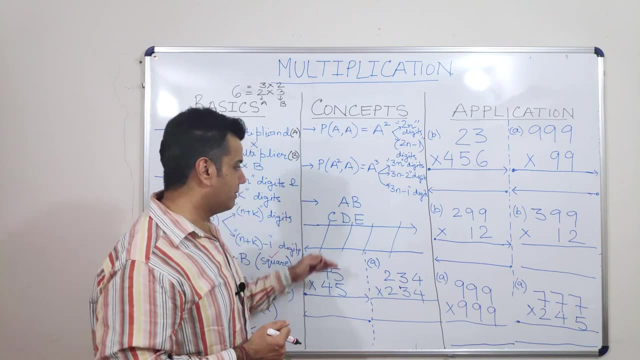 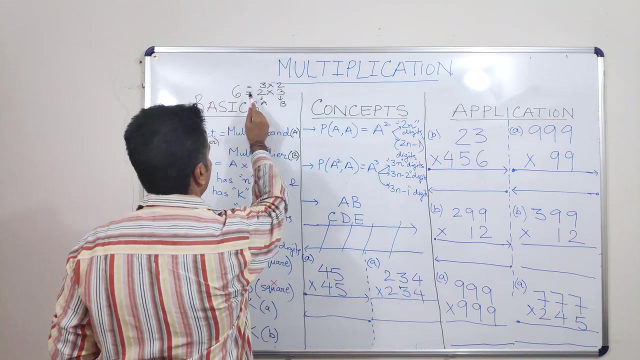 basics to the next level is when i discuss few concepts which are slightly higher than the basics, or the application of the basics only, and then with the help of some examples. okay, so, as the example that i had taken here is, if i take a number like six now i know that 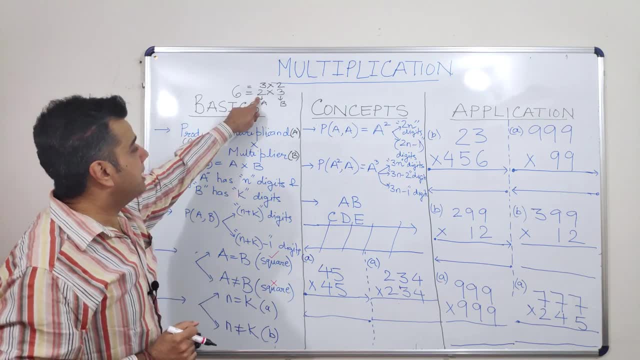 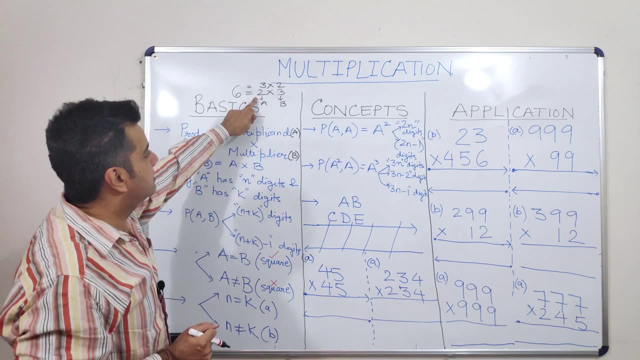 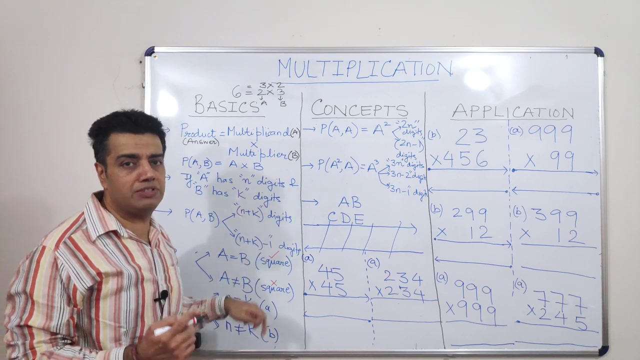 six, if i have written it as two into three. now this number has one digit and this number has one digit, right? so it should give me how many digits. either it should give me one plus one, two digits, or it should give me one plus one minus one, which is one digit only. 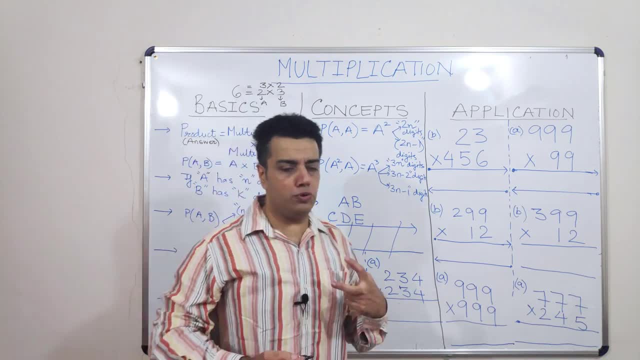 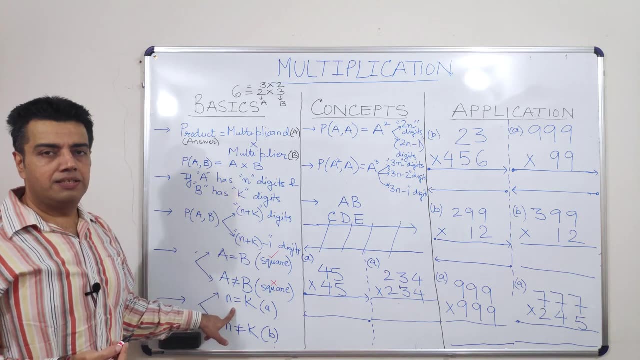 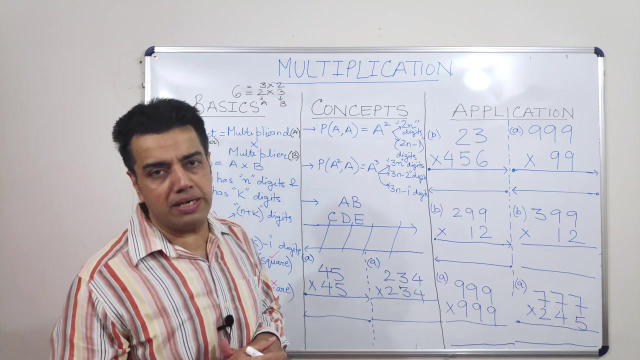 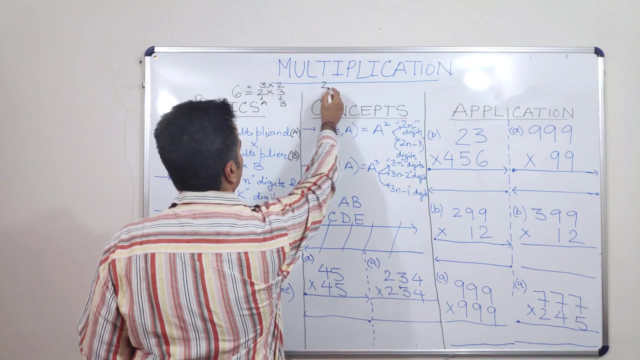 so meaning thereby? if i take the product of two numbers such that both the number numbers had the same number of digits, right, it may give the the. the answer may have either one digit only or it may have two digits. you want some examples here? okay, so can i say two into three gives me a six. 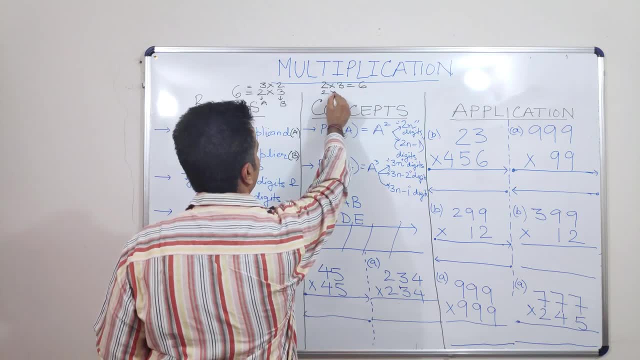 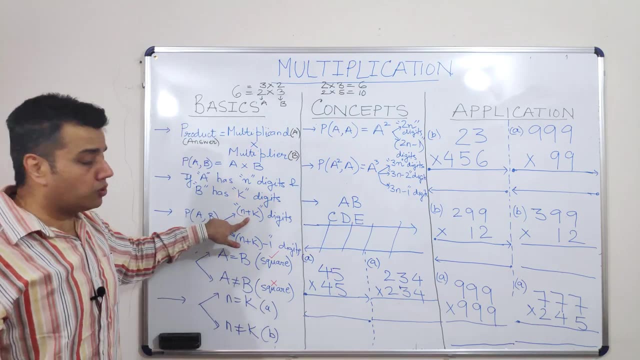 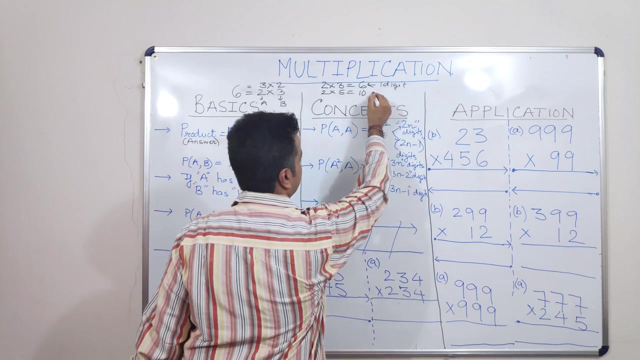 as discussed at the same time. i can say two. 2 into 5 gives me a 10.. Now, this is the case for A. I am sorry, This is what we were talking about. So this has only 1 digit and this has how many digits. This has 2 digits, Meaning. 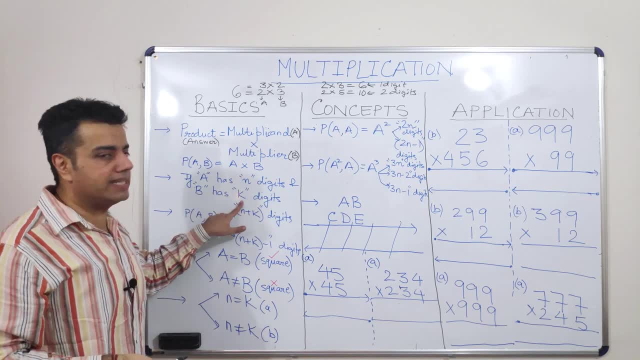 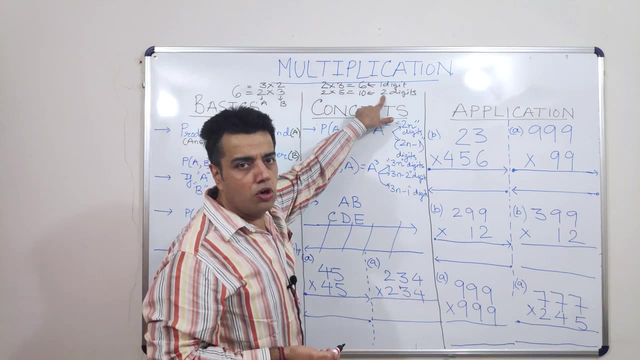 thereby, if A had N digits and B had K digits, now the answer, the product that we are talking about will either have 1 plus 1, which is 2 digits, or 1 plus 1 minus 1, which is 1 digit. 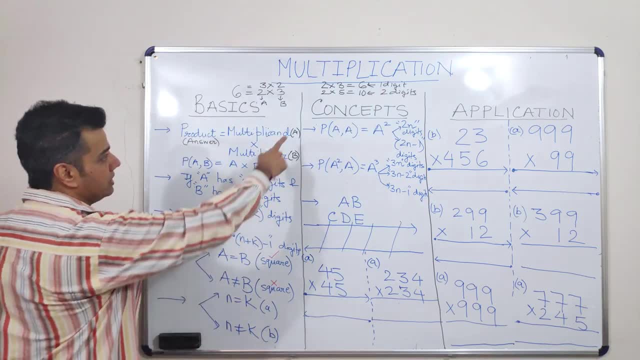 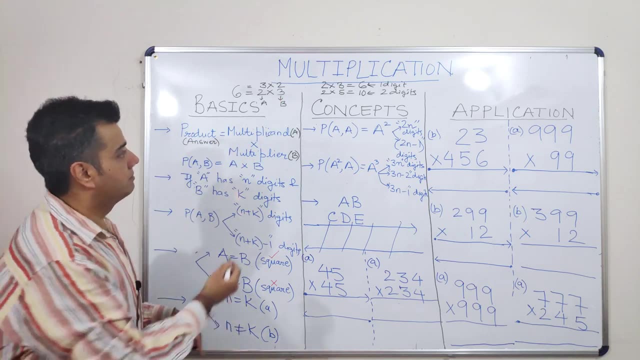 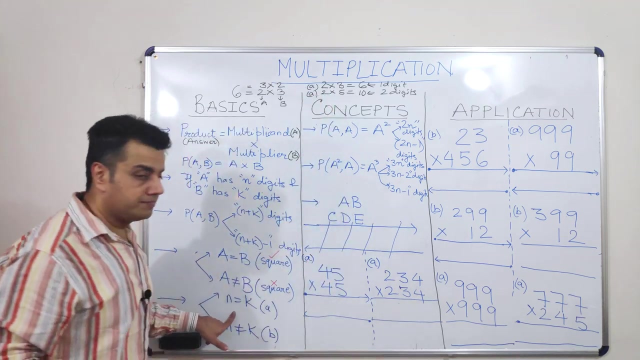 Right. So we took both the examples. So if I were to say which is this example that we had taken, So can I say: here the number of digits are the same And here also, if I would say this is case A. only Now, when I say case A, I am talking about both. 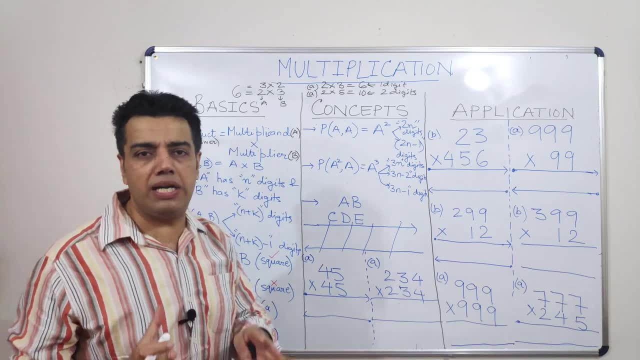 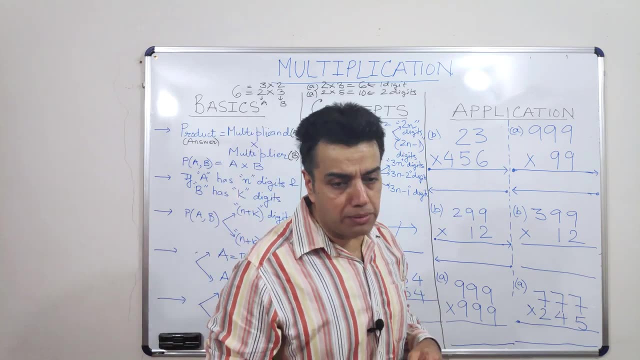 the models. So I am talking about both the models. So I am talking about both the models, The multiplier and the multiplicand having equal number of digits. Taking this to a next level, If somebody tells me that there are 2 numbers which have same number of digits, 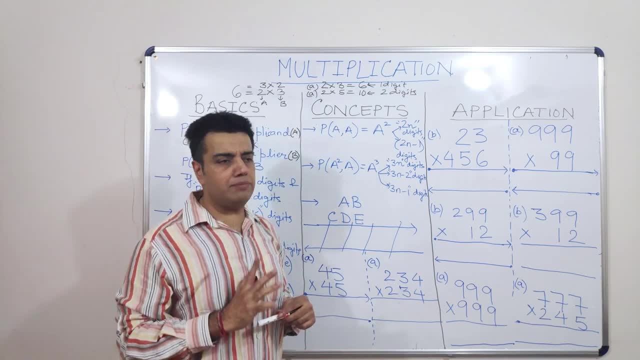 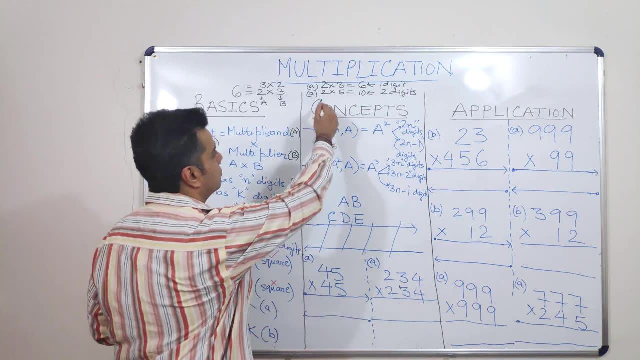 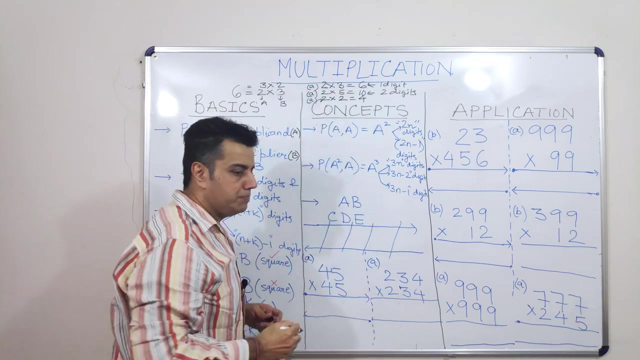 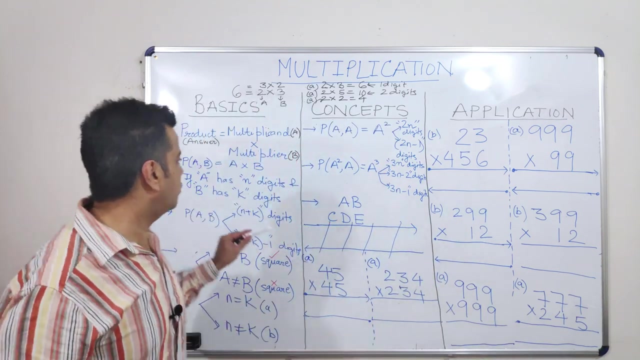 what will I understand? The very first thing that I am going to understand there is: maybe both the numbers are equal, Right, So maybe both the numbers are equal, Maybe both the numbers were unequal. I will repeat: if somebody tells me that I am supposed to find out the product of 2 numbers, 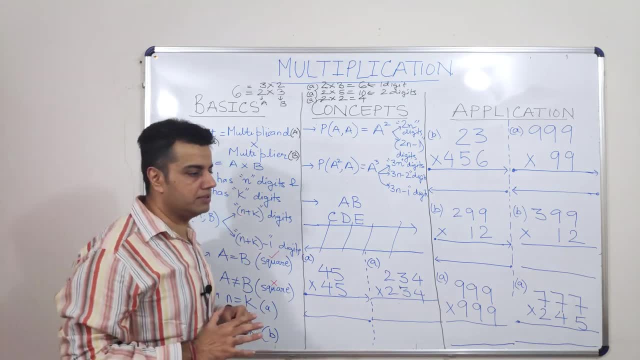 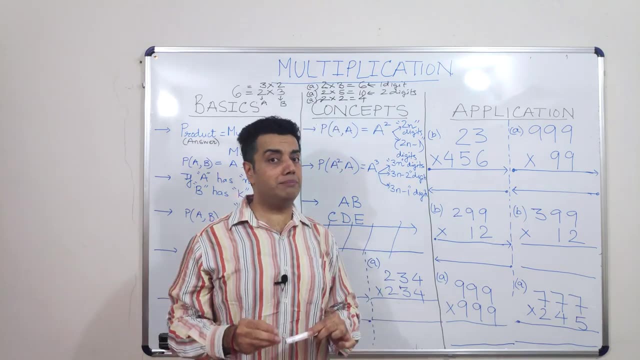 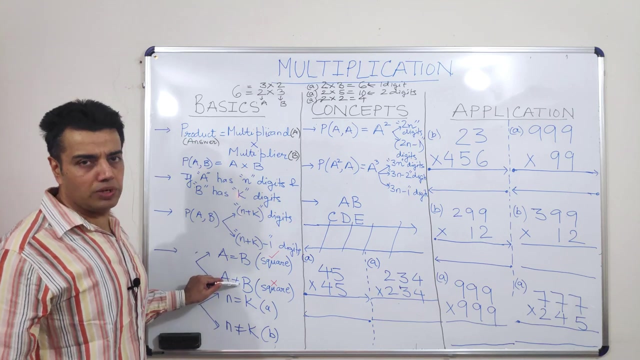 and we are talking about case A, that both the numbers are equal. Now, both the numbers having same number of digits does not mean that both the numbers are equal. So both the numbers may be equal or May be not equal, In case both the number are appear equal. 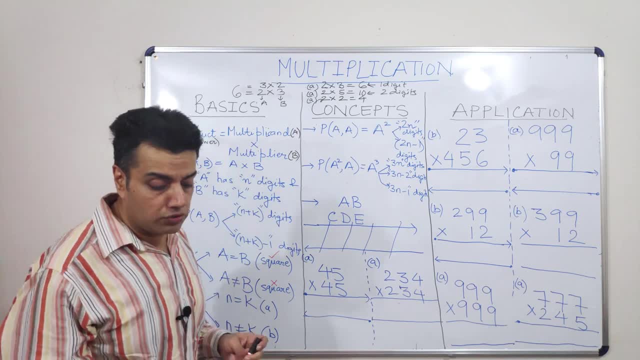 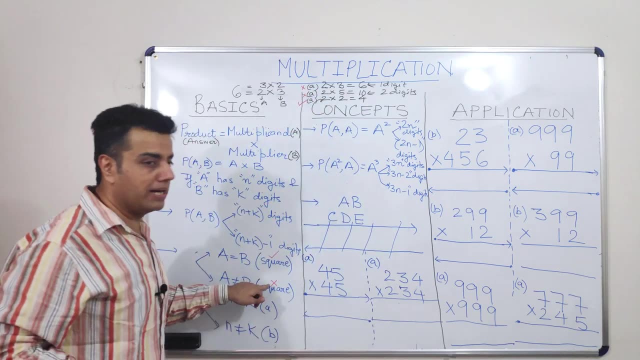 or May not appear equal. Now these numbers are not equal. in case both the numbers, about the numbers, are equal, then we are finding out the square. for example, this case, if both the numbers are not equal, i am denoting it by a cross. cross does not mean that it is incorrect. square means: 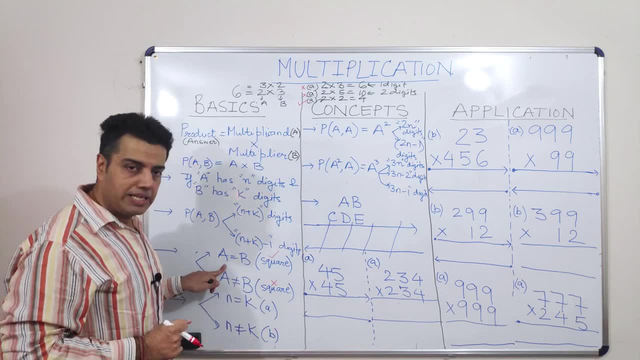 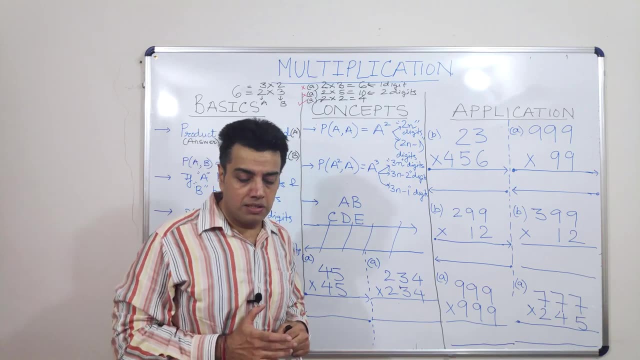 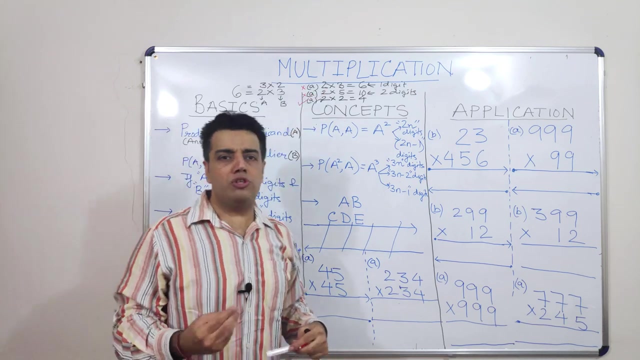 both the numbers are the same. right and cross means that both the numbers are not the same. i hope you understood now. the more you practice in terms of- uh, i mean the examples- that you can take it yourself, and we are starting off with small, small examples only, as you would have seen, 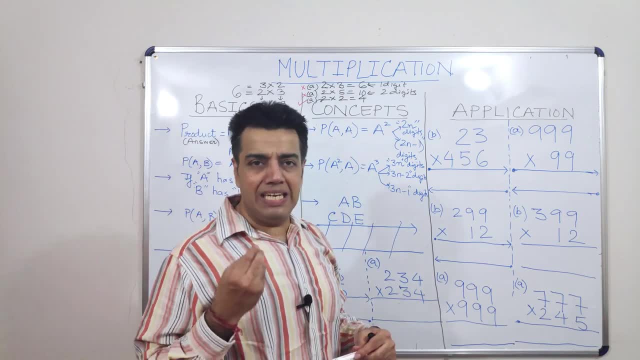 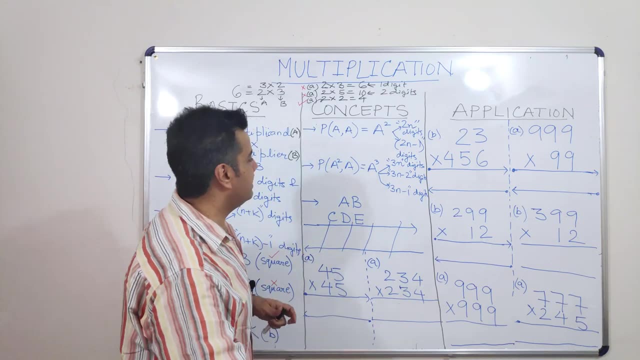 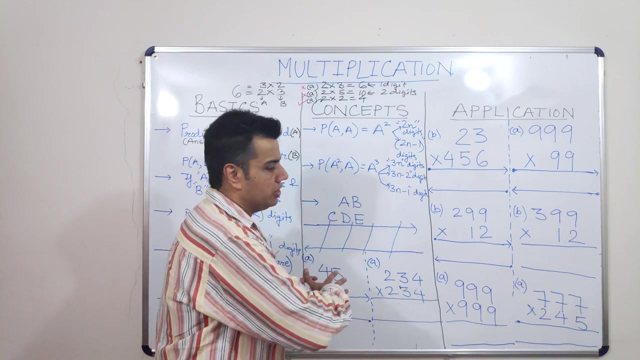 in all my videos, i have always been suggesting: learn big, big things with the help of small examples, right? so the next example that i can take here is: so now if i were to see that what i am going to teach here, have i taught it earlier? no, i haven't. so what have i done earlier if i were? 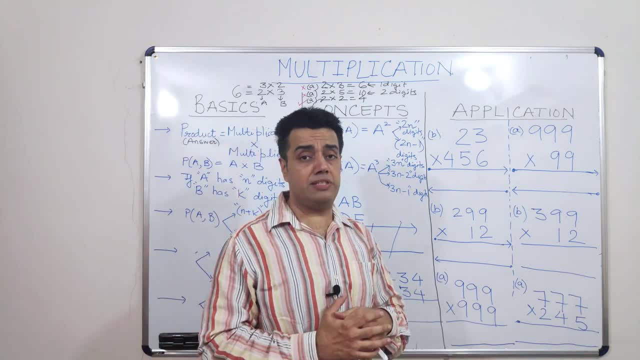 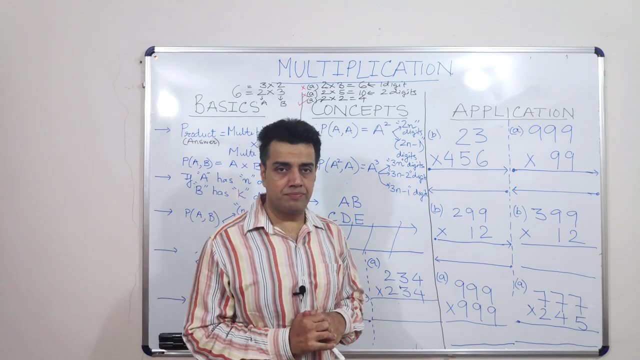 to just revise or if i were to suggest that you should visit. you know, you should see my earlier videos before you do this session. so we have done two digit squares. please relate now, when i say two digit squares, i am basically saying a is equal to b and n is equal to k. 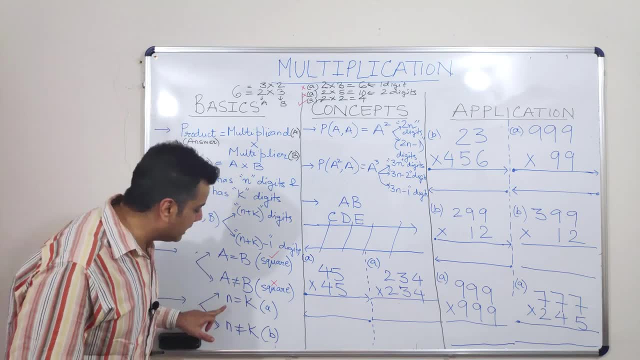 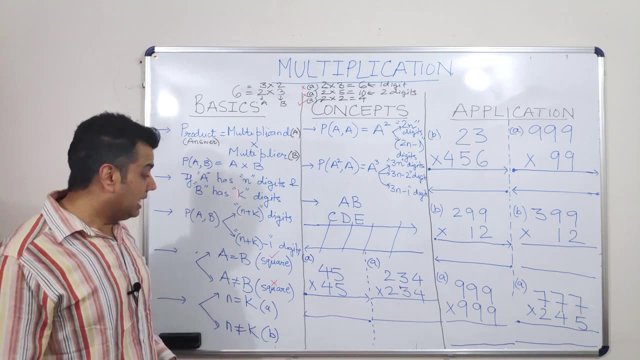 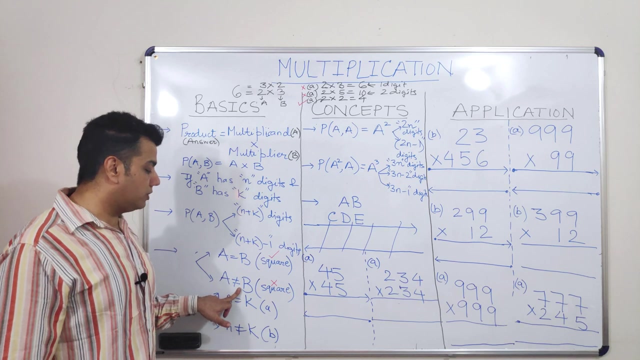 now, when i say three digit squares, i am again referring to a is equal to b and n is equal to k. that means the remaining cases maybe we have not discussed, have we? let us see, we talked about two digit multiplications also. now, if i say a is not equal to b but n is equal to k, so i am basically 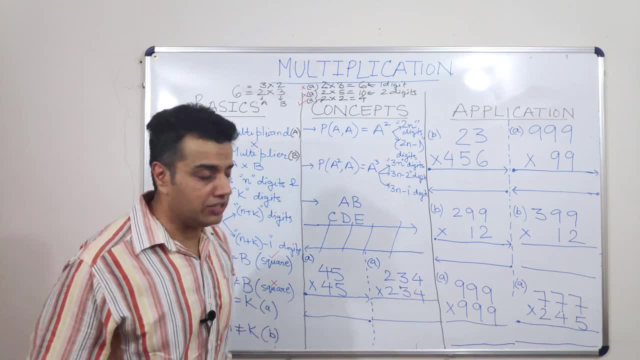 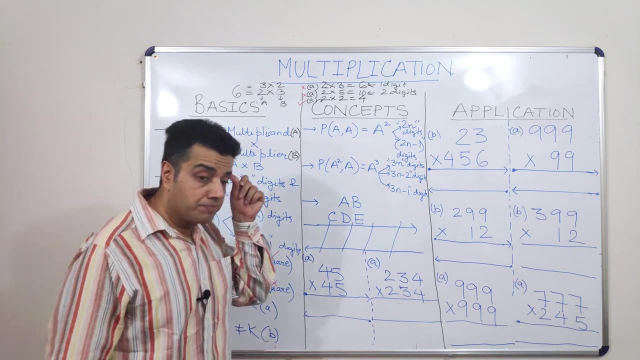 talking about what? let's say, 2 is equal to 2. i am talking about two digit multiplications can have what? either both the numbers may be equal or both the numbers may not be equal. so these are the cases that i have already discussed in my earlier videos. 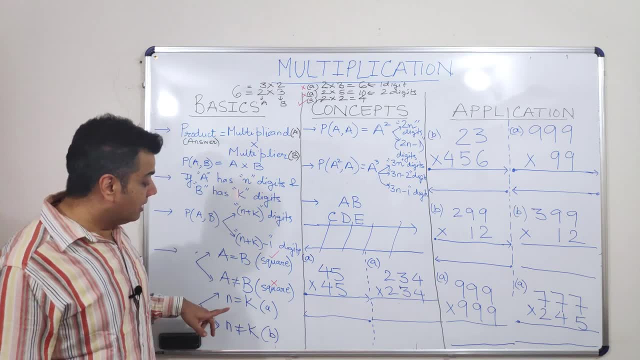 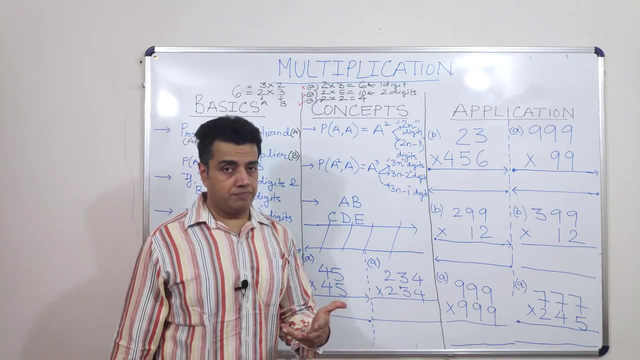 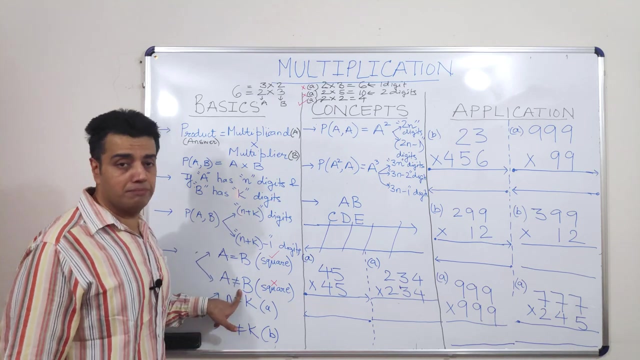 similarly, have i talked about three digit multiplications? yes, which is just like saying both the numbers that i had taken, they had equal number of digits. so i am talking about case a right, but both the numbers may have been the same, may not have been the same, which i have already discussed with you, so please refer to. 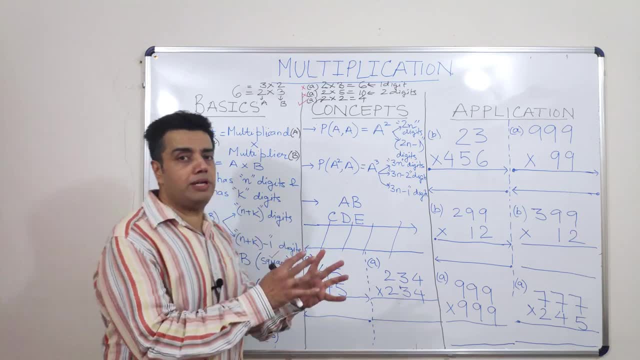 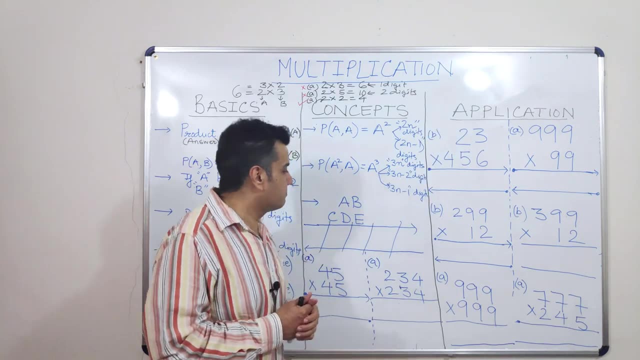 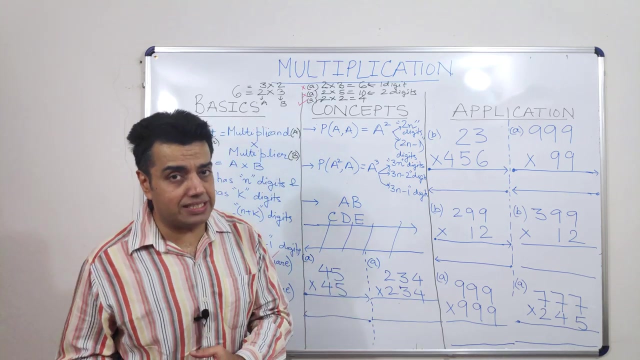 my earlier videos and then combine whatever you would have learnt with this, because knowledge increases as you step up the ladder right. the ones that we have not done are, let us say, a two digit being multiplied with a square, only one digit, or a two digit being multiplied with three digits. 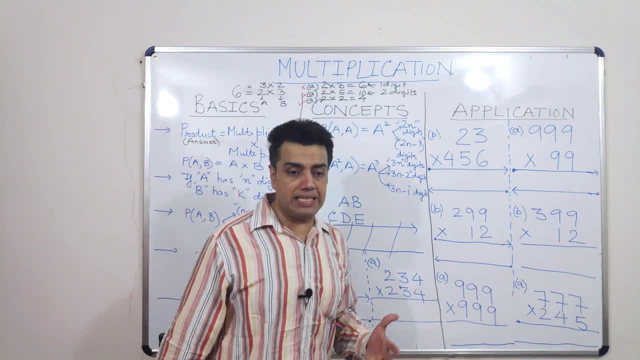 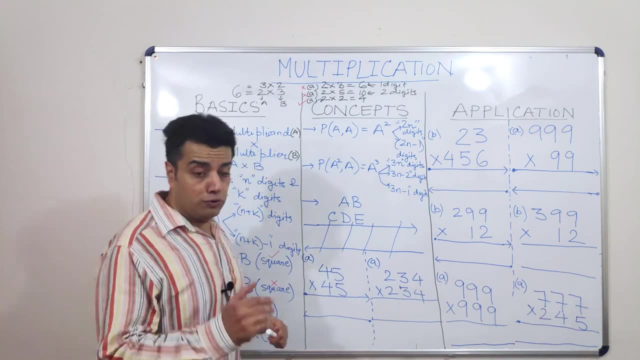 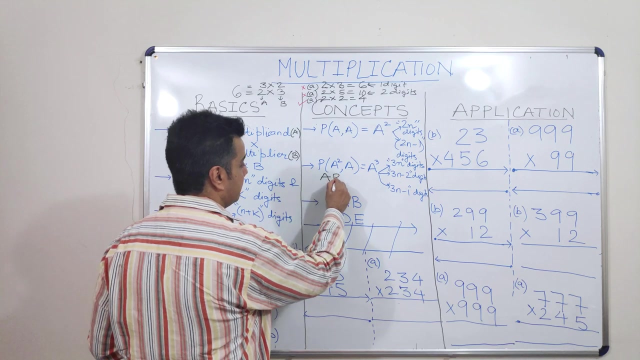 right. so now let us take an example. i am not taking an example of two digit being multiplied by one digit, because i feel that it is a fairly easy example, but if you don't feel the same, let me take one example. so if somebody gives me, let's say there is a two digit number, a, b and i- 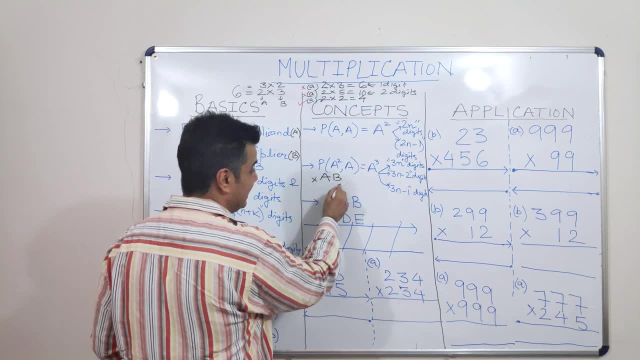 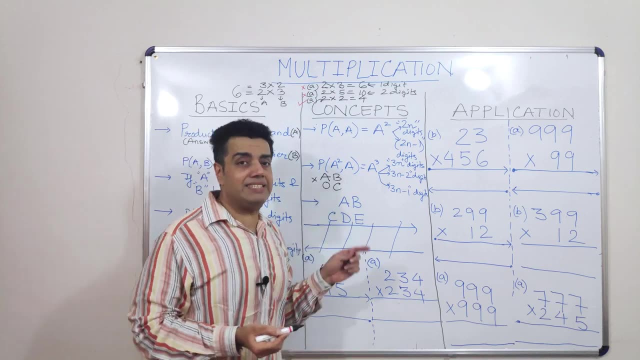 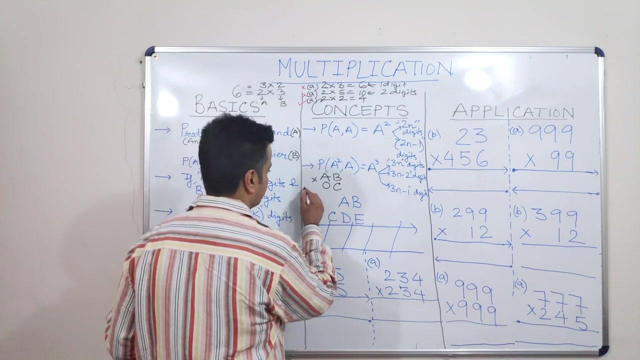 have to multiply it with. multiply it with another single digit, number, c. so if i take a two digit number, of course i can just put a zero here. so this simply gets converted into what a two digit, into a two digit multiplication that we have already discussed. what would be the result here? the result would be a zero. 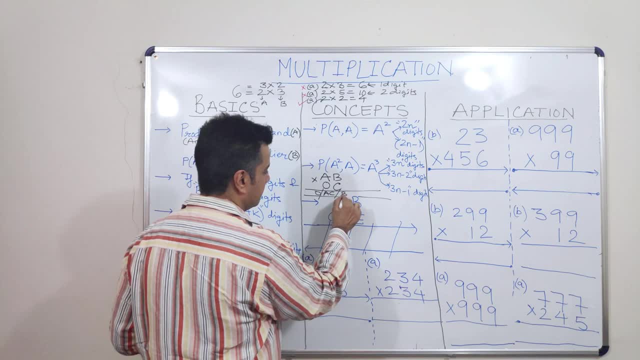 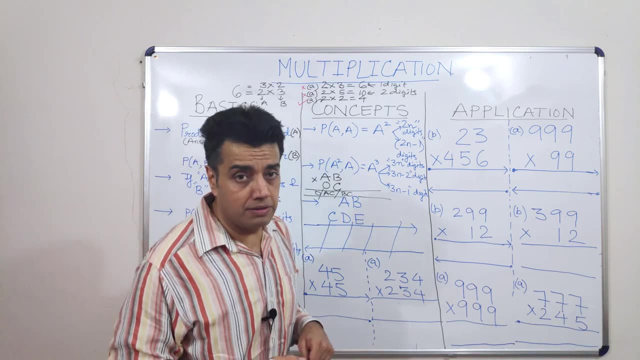 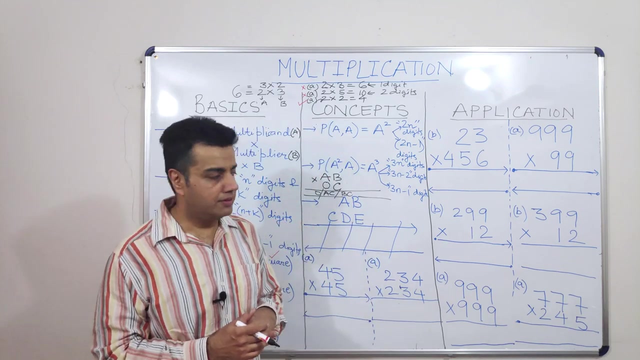 followed by a- c, which is a into c, followed by a- b- c, which is fairly easy. the same logic i am going to apply here, where, if somebody gives me a question like you, have a two digit number being multiplied with another three digit number, what will i do? i will convert both the numbers into three digits only, and i know. 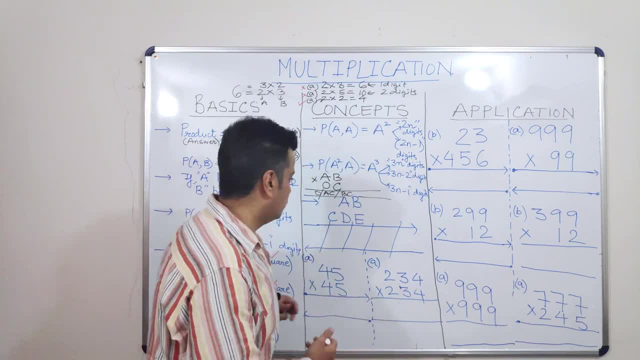 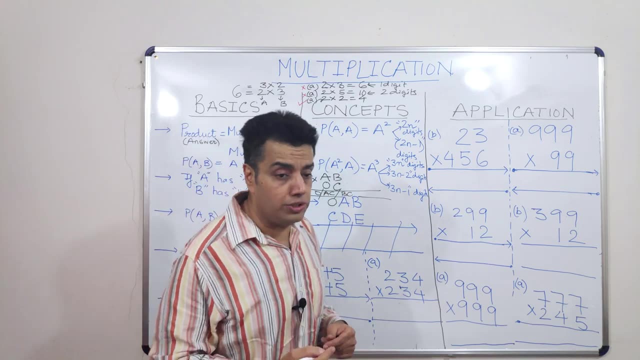 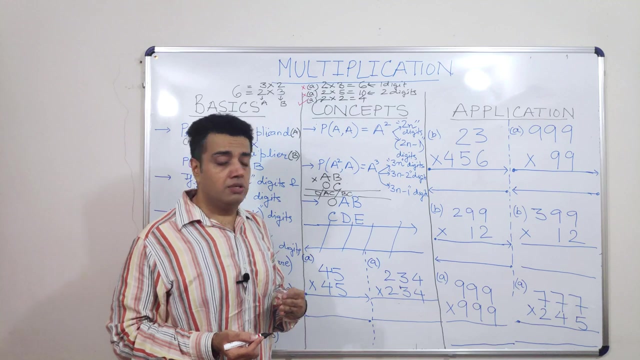 how to multiply two three digit numbers. so what will i do now? this is a two digit number. i'll convert this into a three digit number. now, before doing this, you need to understand that if i put zero before a number, that does not change the value of the number. but if i change, let's say if i put 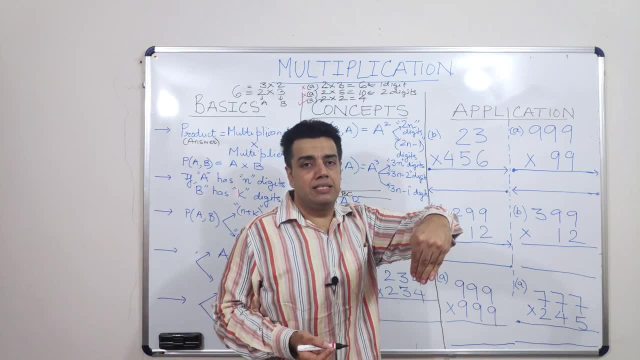 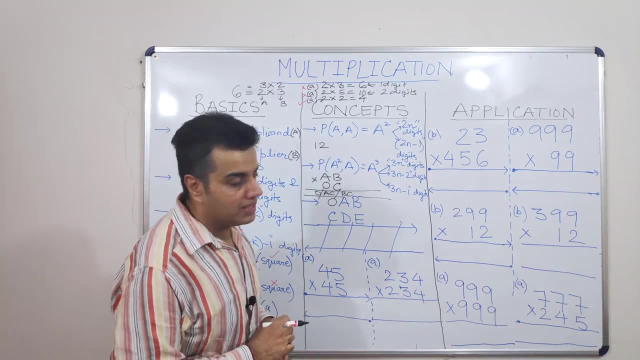 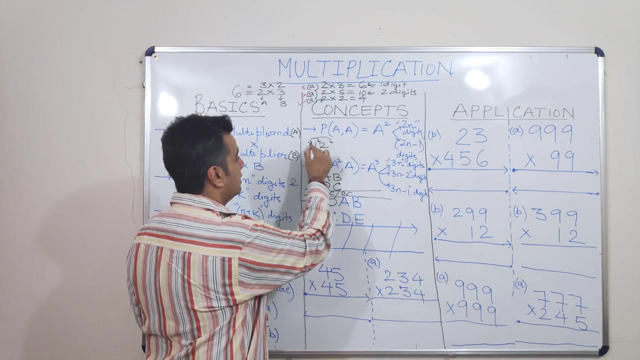 zero after any of the digits or in between any digit, it changes its value. and the best example that you can take here is what if i take a 12 and if i put a zero here, i can put where i can put a zero here. i can put a zero here in between. or i can put a zero here. now, if i put a zero here, it 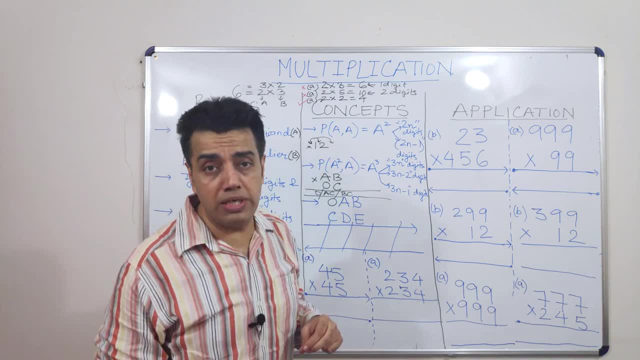 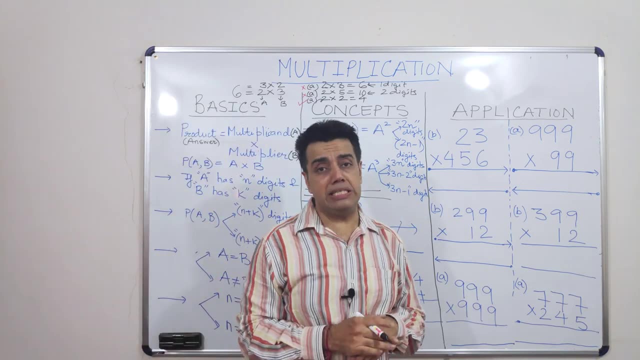 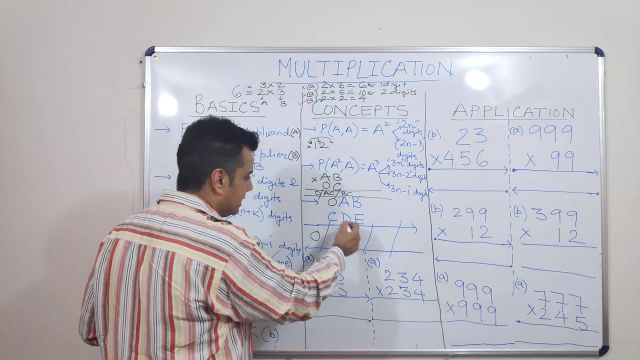 does not make any difference because the number still remains as 12 only. but if i put a zero in between, it changes the number, same with if i put a zero after two, it makes it a hundred and twenty. so, coming back, so this becomes what a zero, followed by you cross, multiply and then you add. 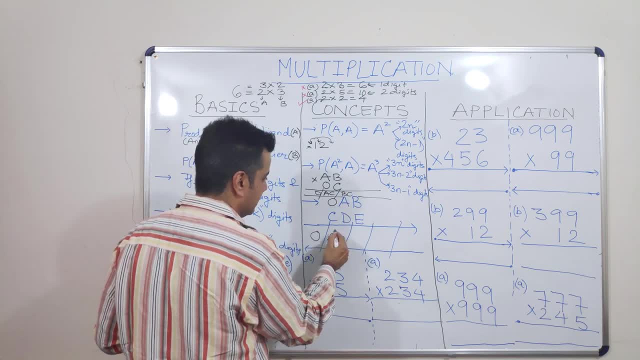 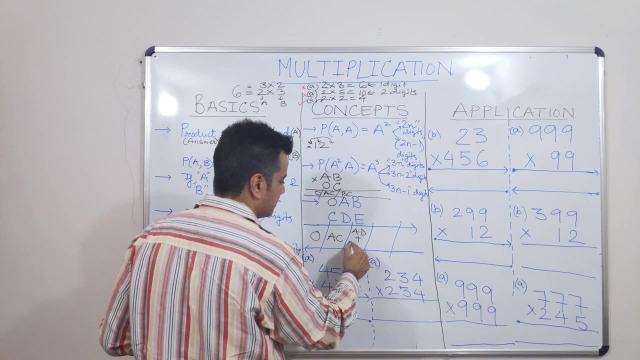 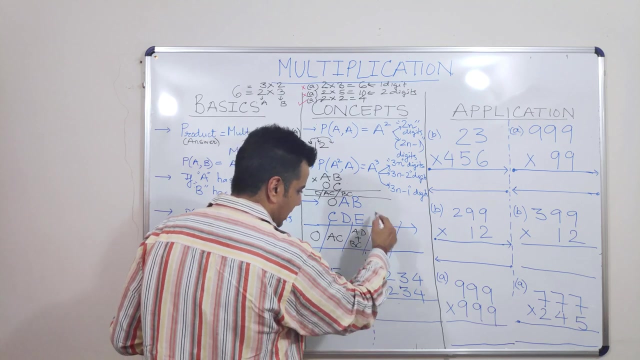 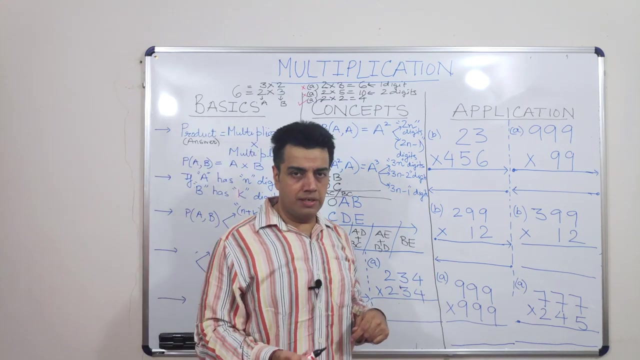 so 0 into d is 0, followed by plus ac, then 0 plus b c plus a d, followed by a e plus b e. sorry, it's b d and followed by b e. okay, fair enough, now we will practice some examples, starting off with an example like: 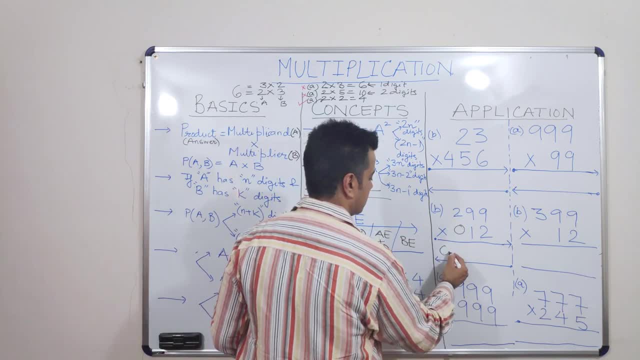 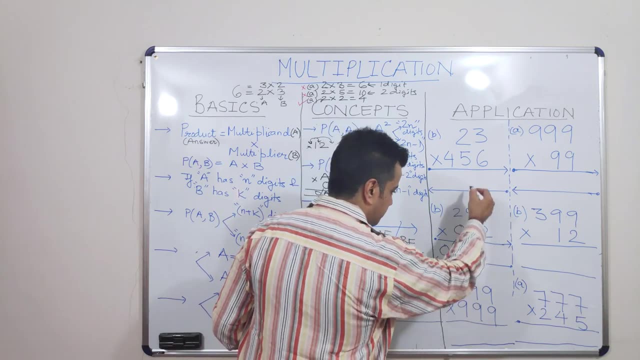 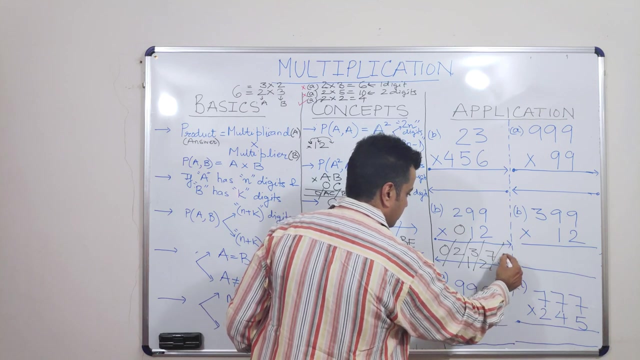 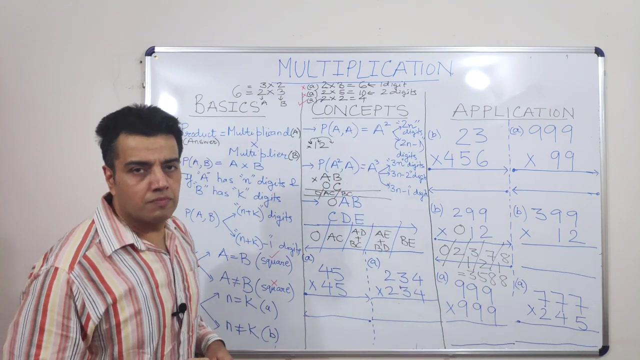 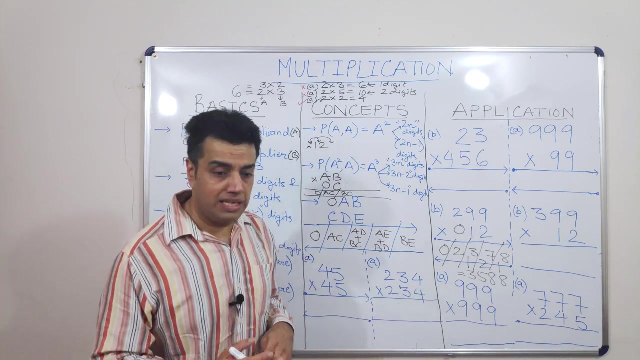 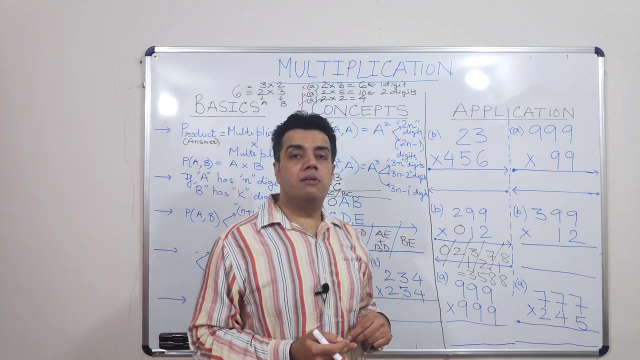 this, so i'm not explaining it to you, because we have already done this in the earlier session, so let us save time here. but then let us revise something that we did, something special in the last video, and in the last video i had told you something like finding the digital roots of a number. let 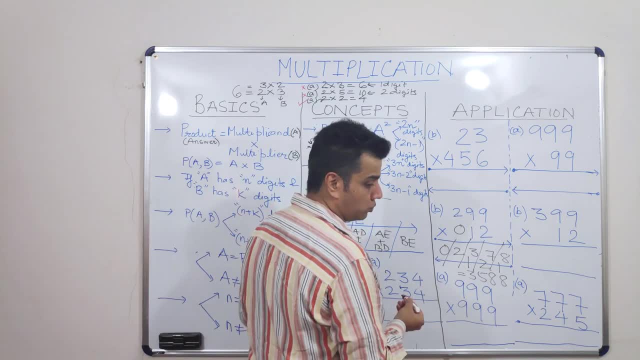 us revise that. so how much is 9 plus 9 plus 2.. it's a 20.. 20 means 2 plus 0.. so the digital root of 299 is a 2.. so it's a 2. so 2 plus 9 plus 9 plus 2 is a 2, so the digital root of 299 is a 2.. 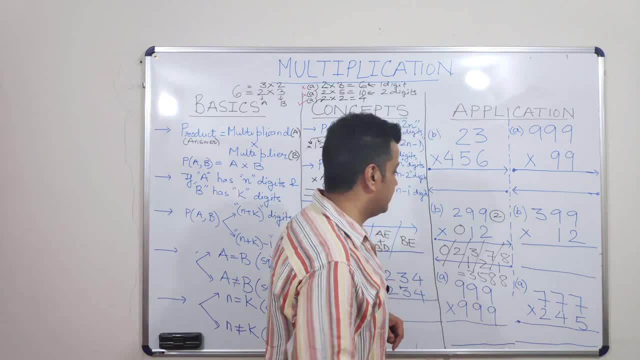 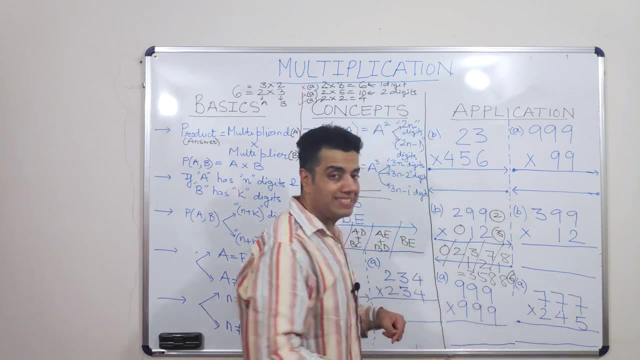 so the digital root of 299 is a 2.. so the digital root of 299 is a 2. right. similarly, what is the digital root for this 3? now, 3 into 2 should give me a 6. let us check whether this is correct or not. 88 plus 8 is a 16. 16 plus 5 is a. 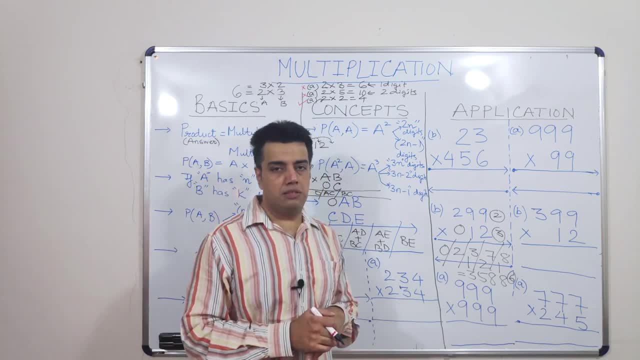 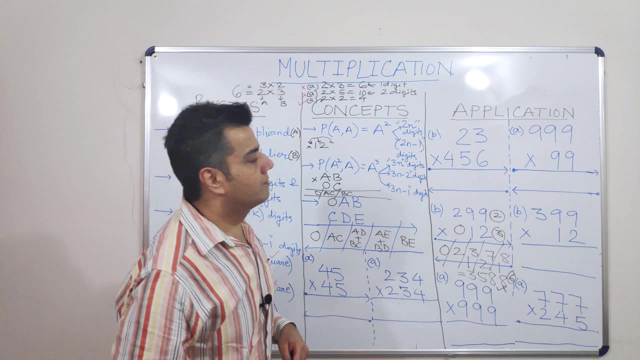 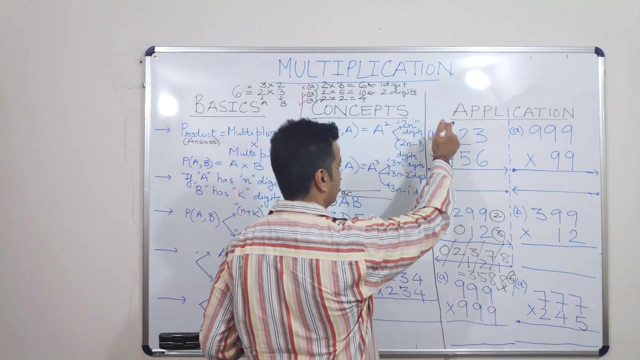 21. 21 plus 3 is a 24. 24, 2 plus 4 is a 6. the answer should be correct. okay, we'll practice one more example, and this time what I have done here is I have slightly changed the orientation. I have taken a two-digit number above, so 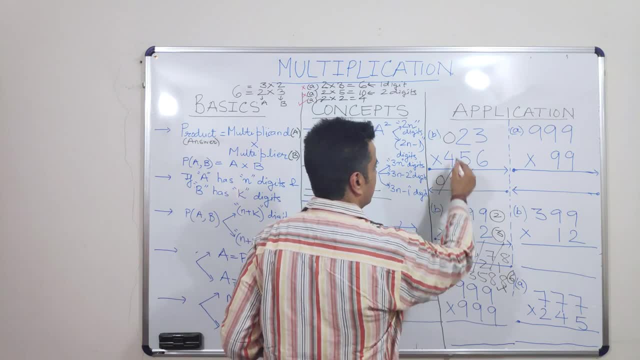 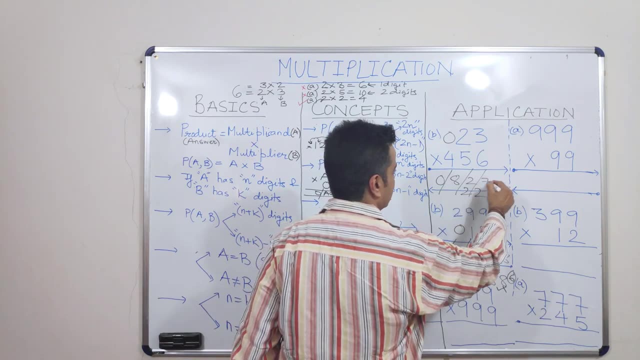 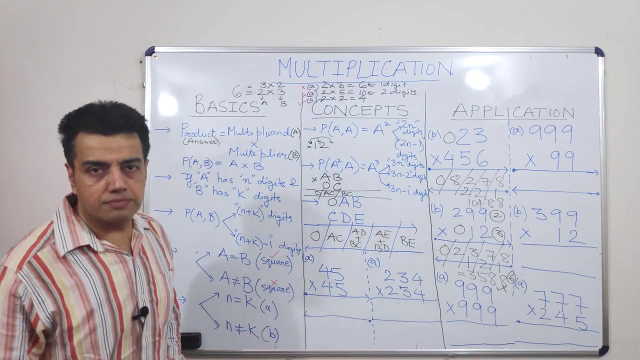 can I say this becomes a 0, followed by 8, 12 and 10 makes it a 22. then can I say 12 and 15 is a 27, followed by 18. so 8, 8, 4. now there are a few things to learn from here. only now this: you will check it for. 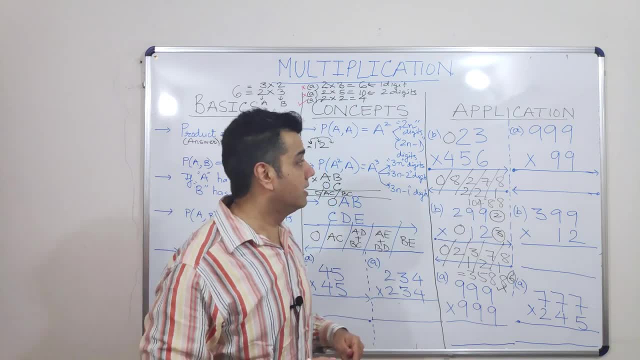 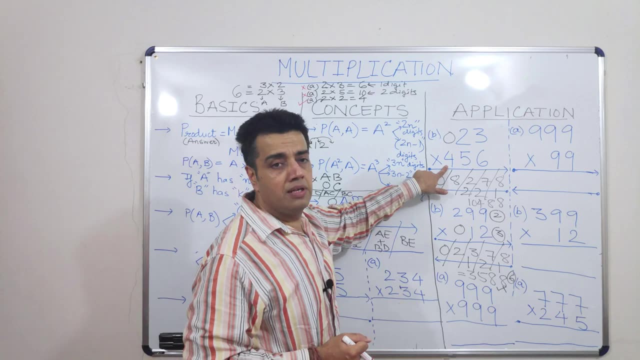 yourself whether the answer is correct or not. you will check it for yourself. whether the answer is correct or not, you'll check it for yourself. you know the method behind it. so let us see this point. we had a two digit number. we had a three digit number, the product of this. 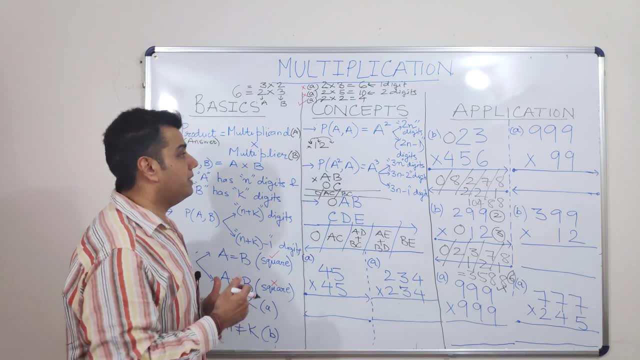 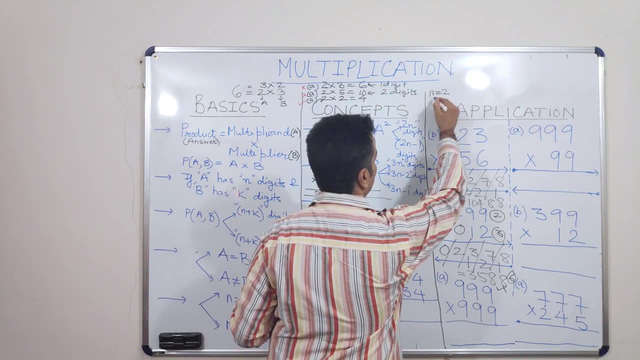 now, this is the product they should give me. how many digits? so if I am taking a two digit number and if I am multiplying it by, so I'm putting it here: if I take the value of n as 2 and K is equal to 3, in that case, how many digits should I? 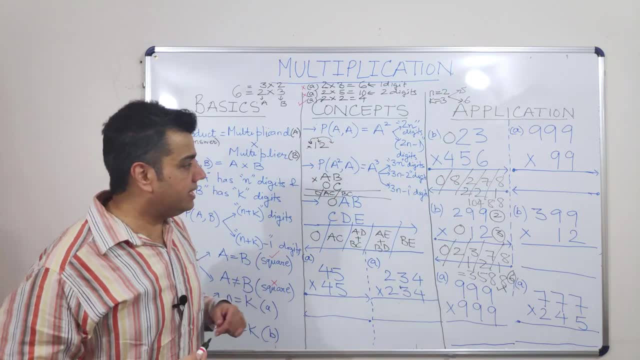 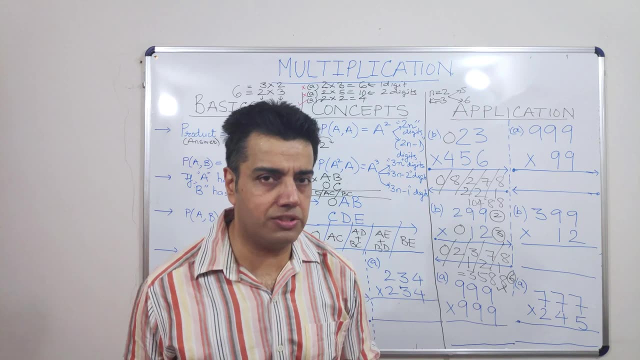 get either 5 or 6 right. so let us see a 2 digit multiplied by 3 digit. how many digits is it giving me? should it give me 5 or 6, or should it give me 5 or 4? so let's revisit. so it should give me 5 or. 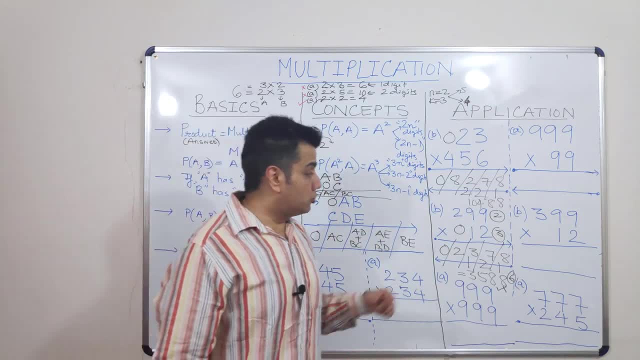 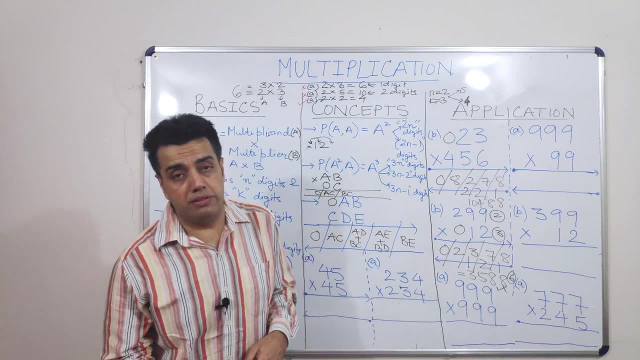 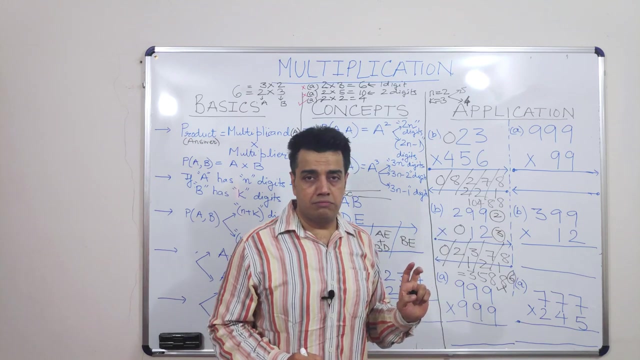 4 digits. so if I multiplied a 3 digit number with a 2 digit number, what is the minimum number of digits that you get can get in the product- 4- and what is the maximum number of digits that you can get- 5. we already got that. similarly, 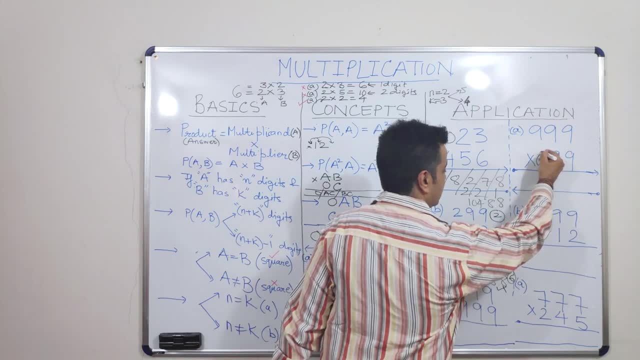 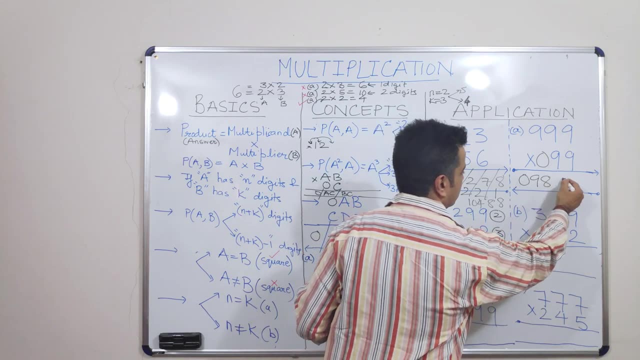 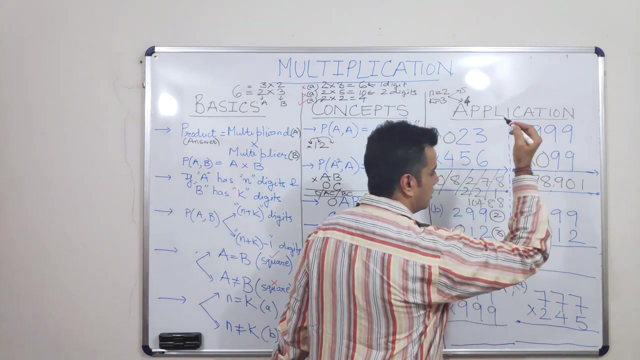 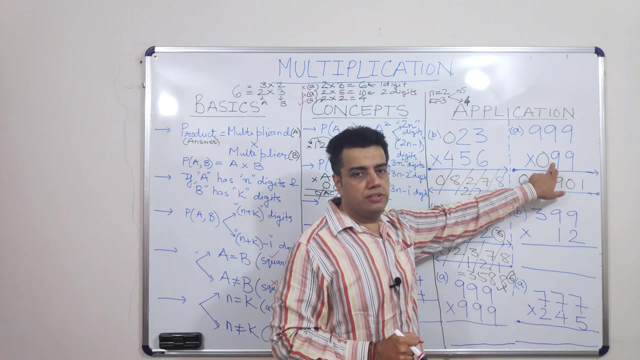 Similarly, this example- I have taken it deliberately because a similar example I had taken in my earlier video, the answer of which is known to you, If you recall now, this had how many digits 3,. this had how many digits 2.. 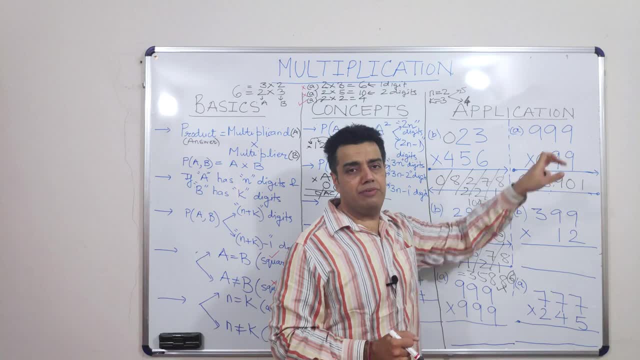 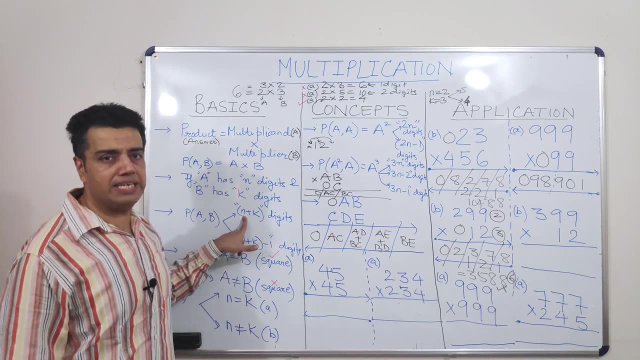 This is the maximum two digit number. This is the maximum three digit number. when I multiply two maximum digit numbers, What is the maximum value that I can get? N plus K digits? Did I get a maximum number of digits here? Now zero will not be counted. 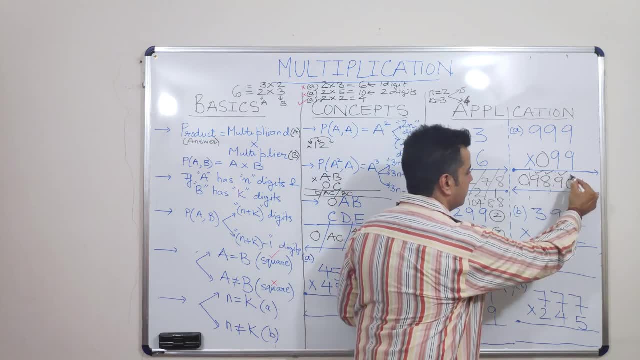 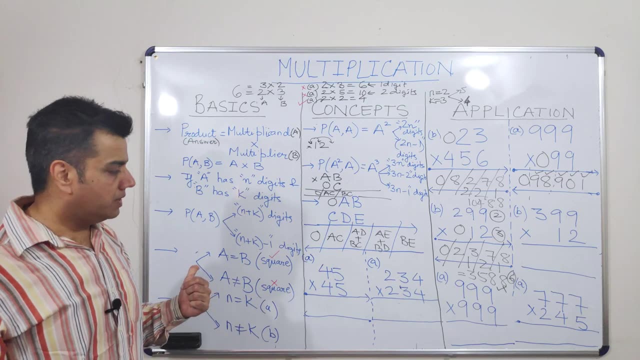 This is just for the sake of understanding. One, two, three, four, five. We got five digits, hence proved: Yeah. Similarly, the last example here and the examples that we are not going to discuss here would be the ones that you would take it as. 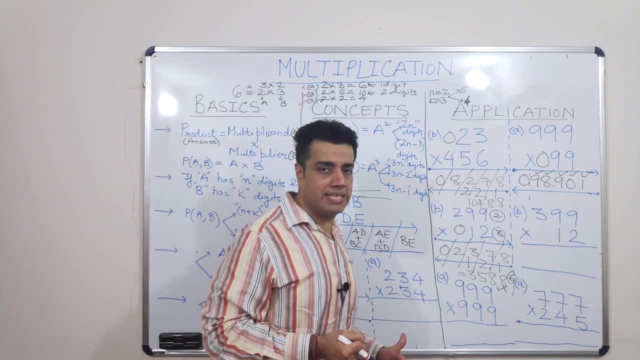 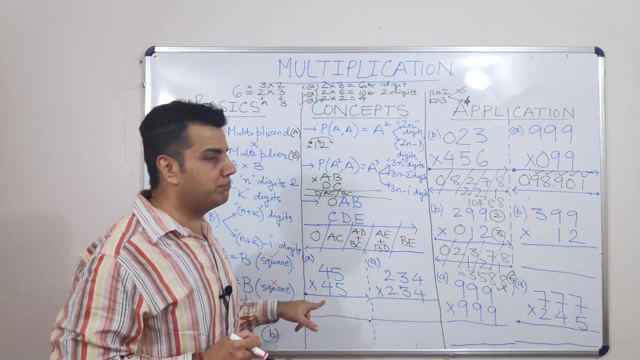 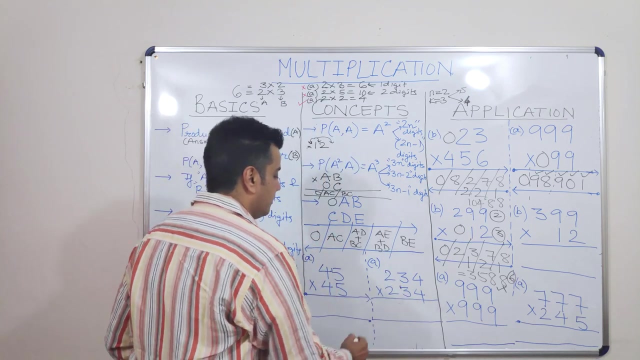 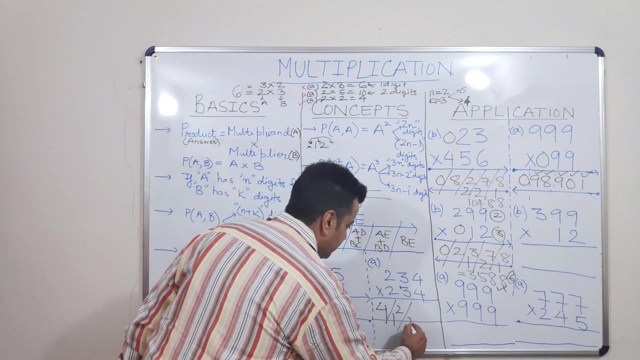 Take home. But you are suggested to solve all the examples once again and whatever is written on this whiteboard, you have to prove each and everything taking those examples, because the examples have been taken very consciously. Okay, So if I were to do this, what will I do for? followed by six and six, 12,, 16 and nine. makes 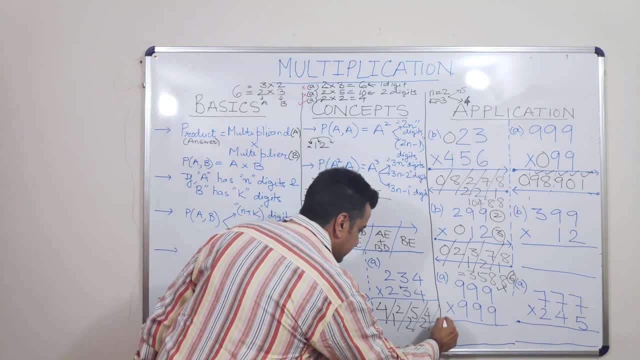 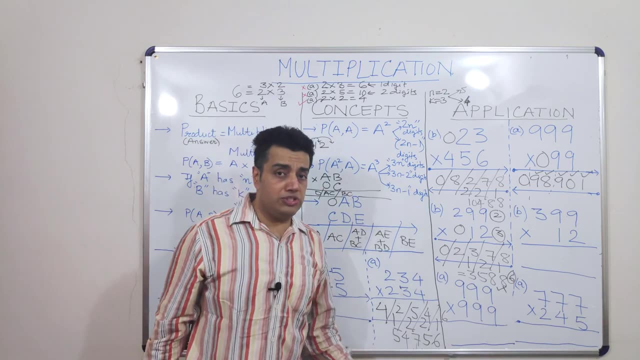 it a 25,, then a 24,, then a 16.. So I should get six, Five, seven, four, and this should be five. The very first thing that you'll do is you'll check whether the answer is correct or not. 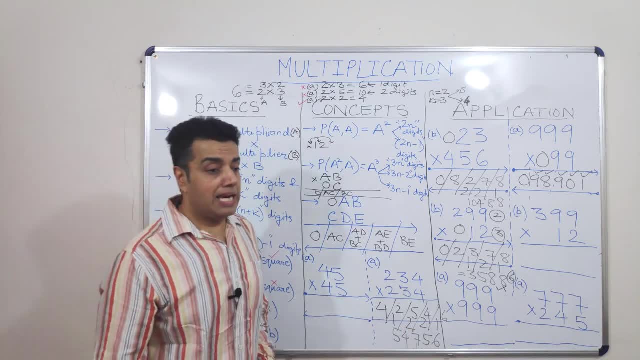 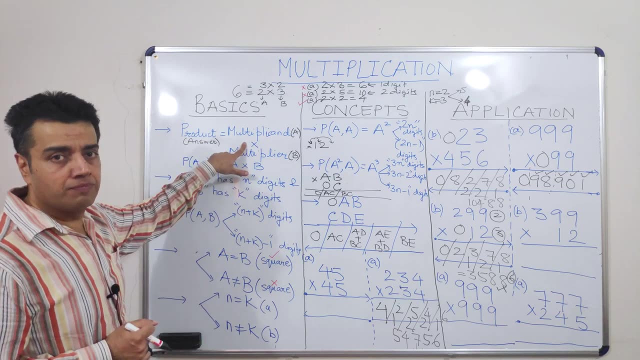 And then, followed by you, will check the number of digits in your answer, And this is what you are supposed to do whenever you're performing any mathematical operation, like multiplication, wherein you are given two numbers. So first you need to get the correct answer. 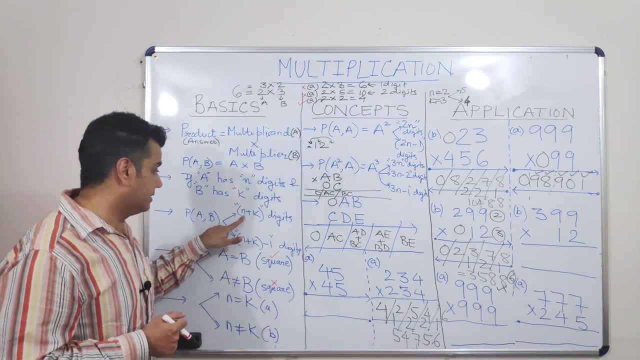 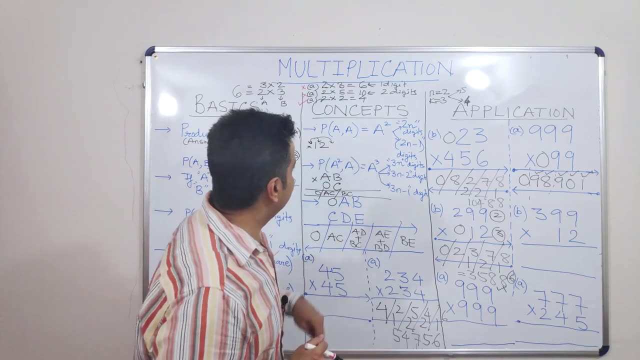 Second, you need to check whether the number of digits were as per these Right Now. the last, but not the least, food for thought for today. Now can I say, if I take both the numbers as same, it is just like saying calculating. 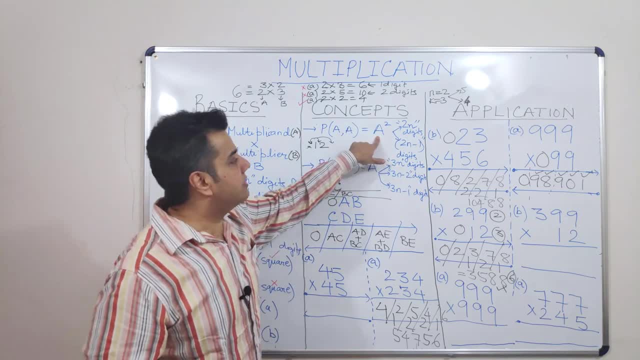 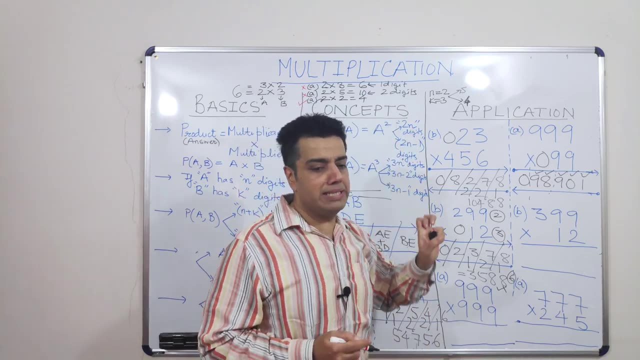 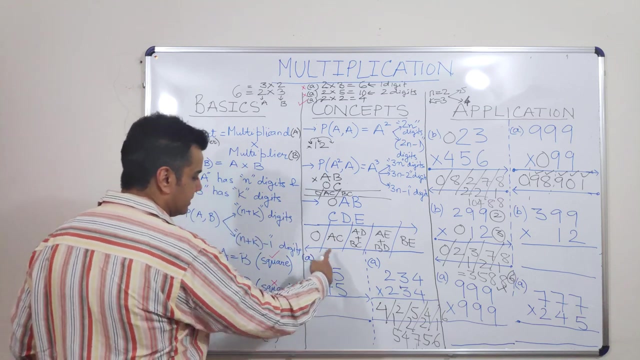 a square right. So if I calculate a square of an end digit number, it'll always give me either two digits or two and minus one. Do we have any example to be discussed from here? Yes, We can take this as an example. 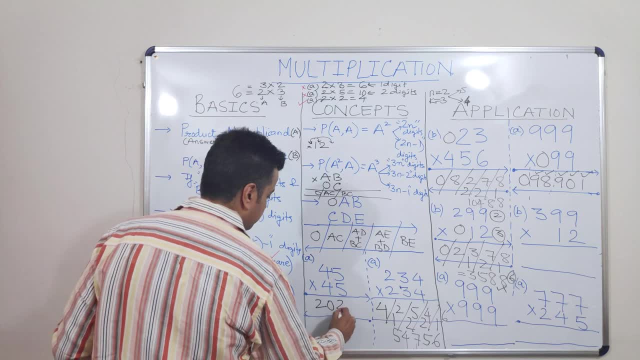 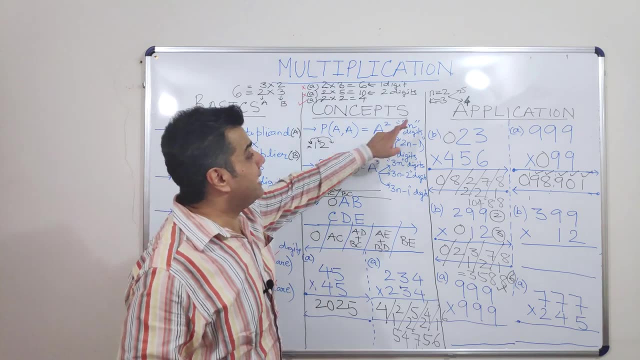 Now, how much is 45 square? We can always find it out. Now, this had two digits right And it is giving me how much N plus N. If you recall, it can give me a maximum of N plus N, which is just like saying: 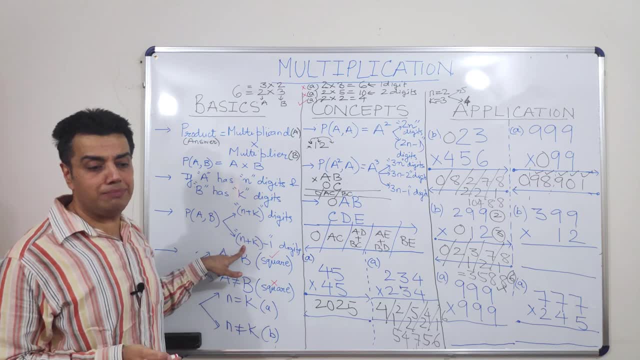 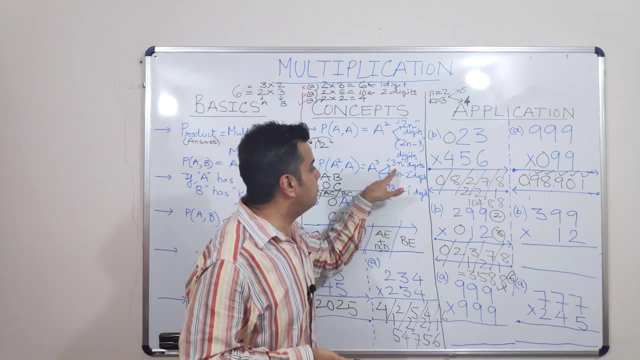 what two N digits and a minimum of how much N plus N minus one, which is just like saying two N minus one digits, proved. the same thing I can say for cubes, But here one more possibility increases. So we'll talk about this when we talk about in one of my videos.